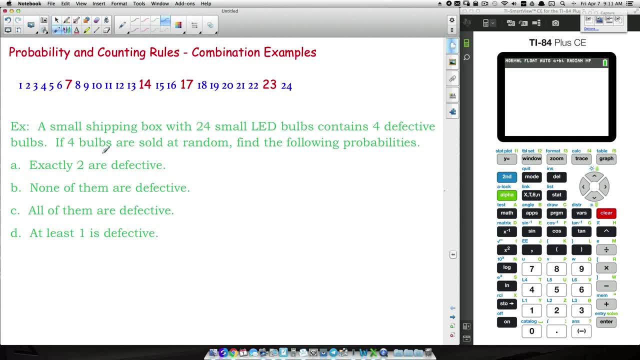 notice. the example says we have four defective bulbs out of 24, and we're going to sell four of them at random. Now the reason why this is a combination. suppose you sold to a customer. this could be like at Radio Shack or some electronic store where they have LEDs. 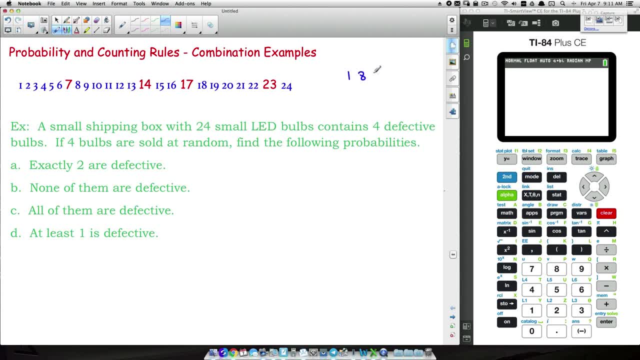 Suppose you sold a customer bulb 1,, bulb 8, bulb 14. Whoops. So bulb 1,, bulb 8,, bulb 14. Well, we don't know it, but I'm just pointing it out- And then bulb 19.. Okay, That's one possible way to sell four bulbs to a customer, right. 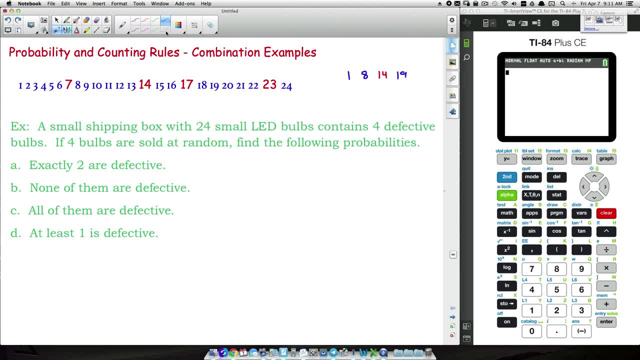 Well, here's the point. A combination is when order does not matter. So is this going to be the same sale to a customer? Answer this question right here. If we sell them bulb 8,, bulb 14,, bulb 1, and bulb 19, isn't that the exact same four bulbs right? 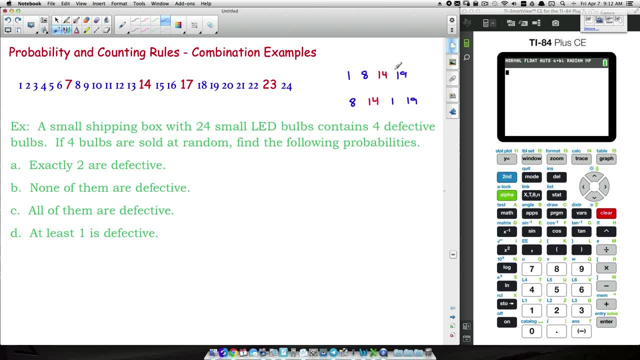 It's just like the order in which you pull them off a shelf. It does not matter If you sell a customer these four bulbs. it's the exact same thing as selling them these four bulbs. So the order does not matter, And that's why this is a combination Permutations. order does matter, But 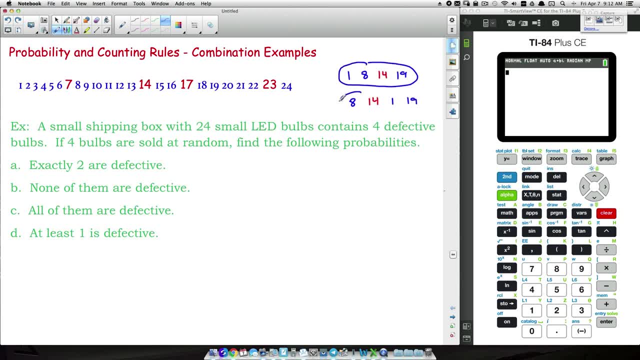 here, selling a customer. this is the exact same thing as selling a customer this. And once you get that concept down, then you can start applying your combination rules. But again, permutations- we'll address that in a future video, But right now we're dealing with combinations. 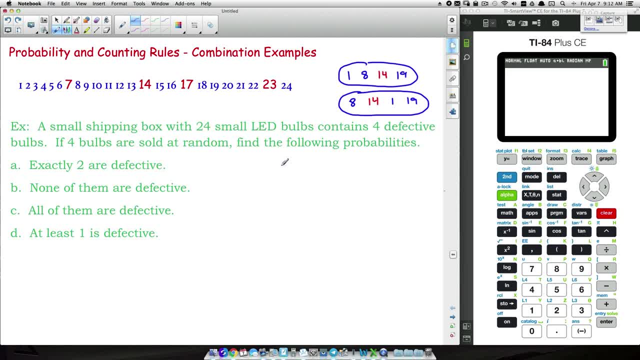 So let's just write down a few facts. We got four defective and we have 20, let's call them working. 20 of them work because we have 24 bulbs in all. right Now, let's address some other things too. Well, how many ways you know this right here. this is not two ways, This is one way of. 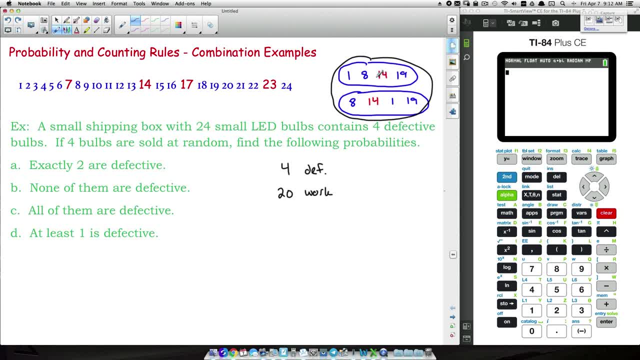 selling four bulbs to a customer Because, again, order does not matter. Well, how many ways can we do this? How many ways can we sell four bulbs to a customer? How many ways can we sell four bulbs to a customer? How many ways can we sell four bulbs to a customer? How many ways can we sell four bulbs? 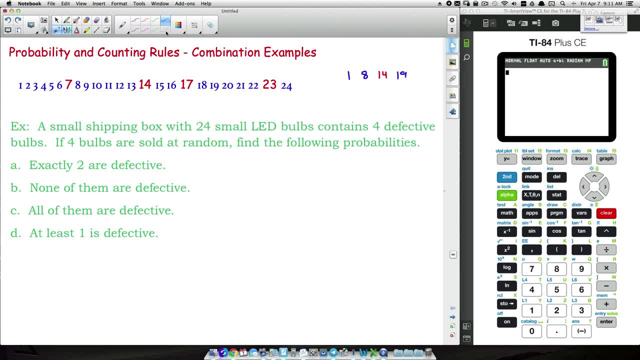 Well, here's the point. A combination is when order does not matter. So is this going to be the same sale to a customer? Answer this question right here. If we sell them bulb 8,, bulb 14,, bulb 1, and bulb 19, isn't that the exact same four bulbs right? 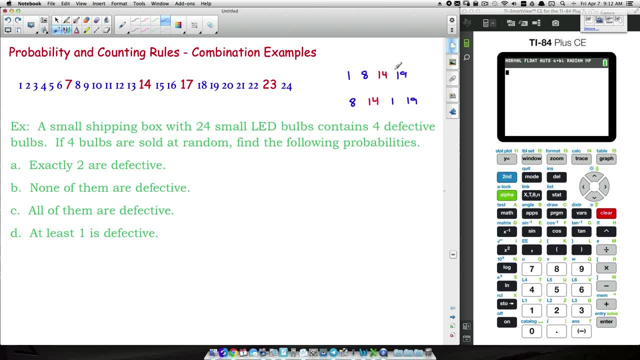 It's just like the order in which you pull them off a shelf. It does not matter If you sell a customer these four bulbs. it's the exact same thing as selling them these four bulbs. So the order does not matter, And that's why this is a combination Permutations. order does matter, But 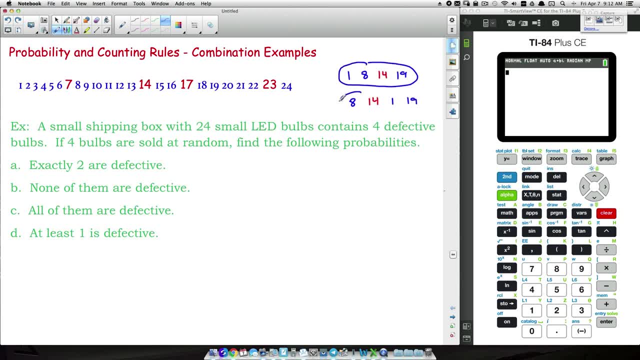 here, selling a customer. this is the exact same thing as selling a customer this. And once you get that concept down, then you can start applying your combination rules. But again, permutations- we'll address that in a future video, But right now we're dealing with combinations. 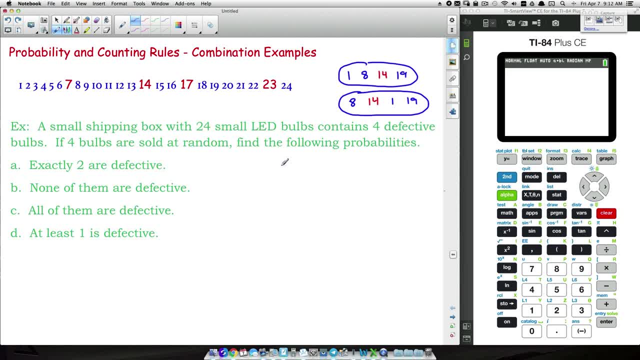 So let's just write down a few facts. We got four defective and we have 20, let's call them working. 20 of them work because we have 24 bulbs in all. right Now, let's address some other things too. Well, how many ways you know this right here. this is not two ways, This is one way of. 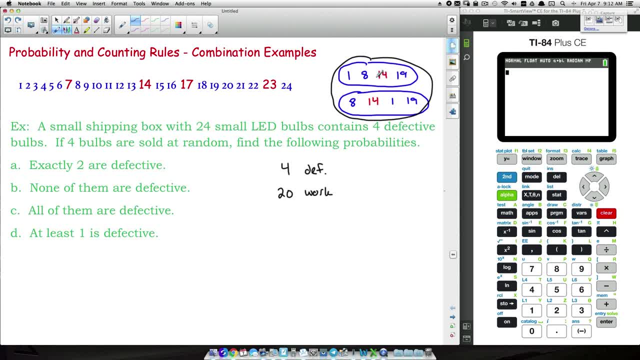 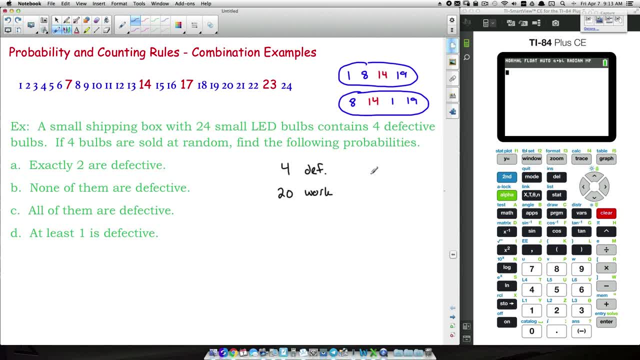 to a customer. Well, that's going to be used in pretty much all these problems. So, out of 24 bulbs, how many ways can we sell four of them? And since we said it's a combination, this right here is going to be the total number of ways that you can sell four bulbs to a customer out of the 24 bulbs. 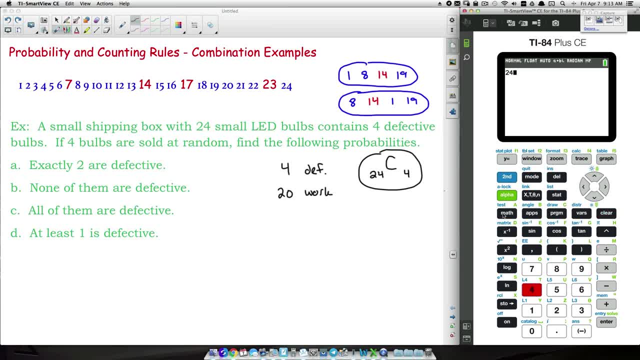 So let's go ahead and figure that out: 24, on a TI-84,, we go 24, press math, go over to prob and we want to do a combination. So three, So 24, we want to choose four because we're selling. 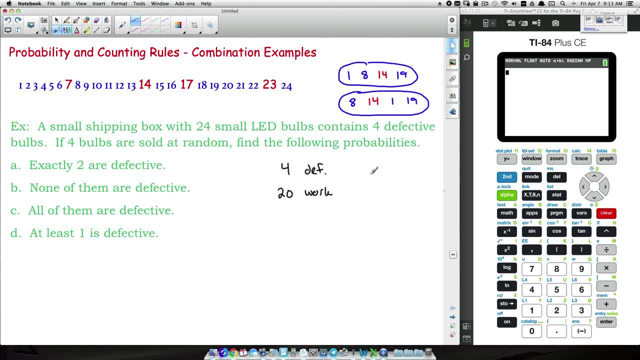 to a customer. Well, that's going to be used in pretty much all these problems. So, out of 24 bulbs, how many ways can we sell four of them? And since we said it's a combination, this right here is going to be the total number of ways that you can sell four bulbs to a customer out of the 24 bulbs. 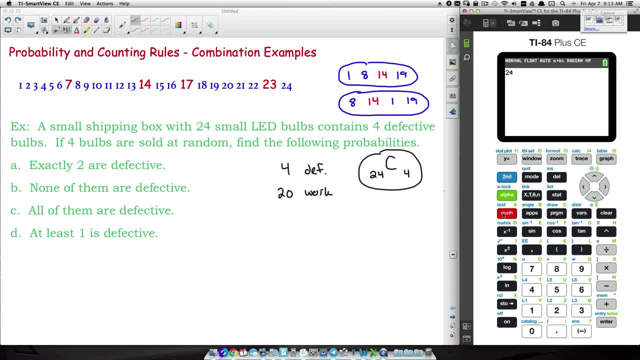 So let's go ahead and figure that out: 24, on a TI-84,, we go 24, press math, go over to prob and we want to do a combination. So three, So 24, we want to choose four because we're selling. 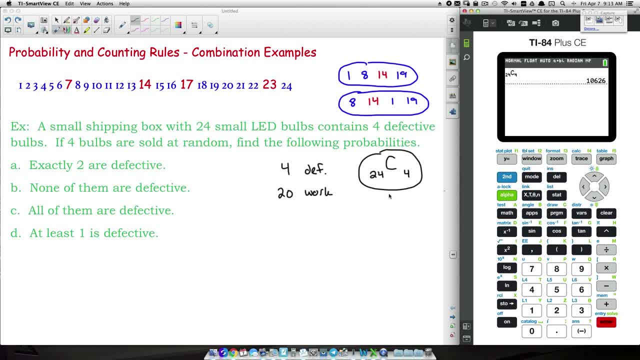 four bulbs. So we have a total of 10,626 ways, 10,626 ways that you can sell four bulbs out of 24 bulbs to a customer. And again, this right here, that's just one way, because again, order does not. 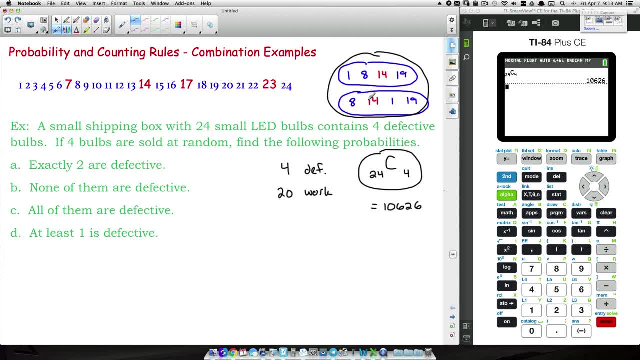 matter. in a combination We're still selling the same four bulbs. I hope that makes sense there. So how can we sell exactly two bulbs? Well, let's think about that. Question A: we're trying to sell exactly two bulbs. Question B: we're trying to sell exactly two bulbs. Question C: we're trying 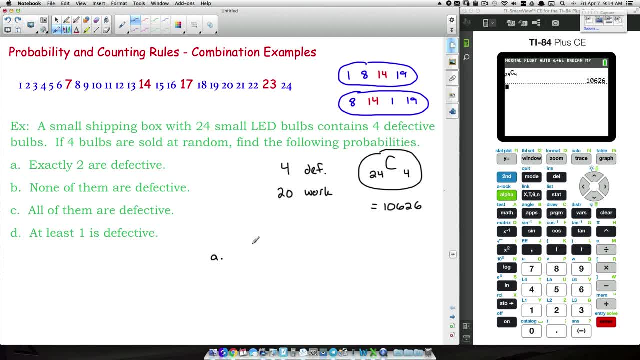 to sell exactly two. Well, let's think about this. How many ways can you do that if we look at the defective, Out of four defective bulbs, we want to choose two of them because we want exactly two. Notice, I'm picking the four here. So four choose two. The reason why I'm doing that: 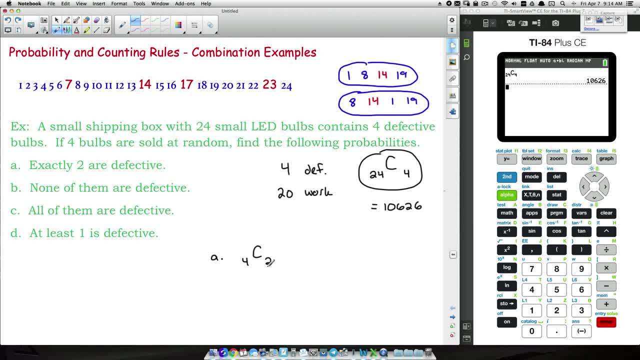 is because, out of the four defective, I want to choose any two of them. Now again, that would be no different if I said okay, if I picked bulb 14 and 17,, if those were sold in a set of four. 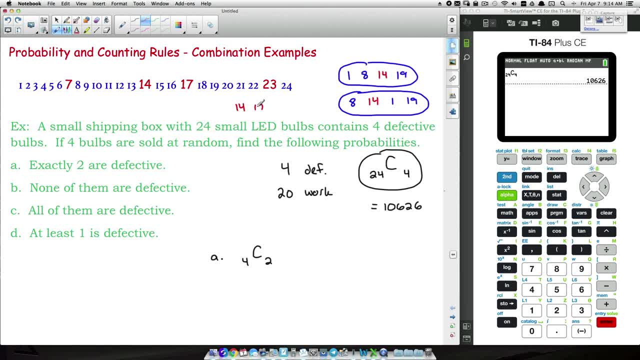 selling 14 and 17 would be the same thing as selling 17 and 14, because it's still the same two bulbs. Order does not matter. Well, those are our two bulbs. Well, how many are we selling in all? We're selling four bulbs in all, So there's still two bulbs left that we're going to sell. 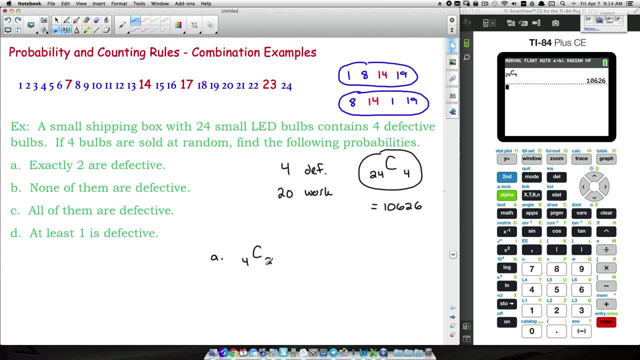 So what do we do here? Well, we're selling four bulbs. Two of them are going to be defective. That's going to leave the remaining two that are going to be working fine. Well, how many ways? what are we choosing from here? It's going to be 20 working. Now think about this. Out of four of 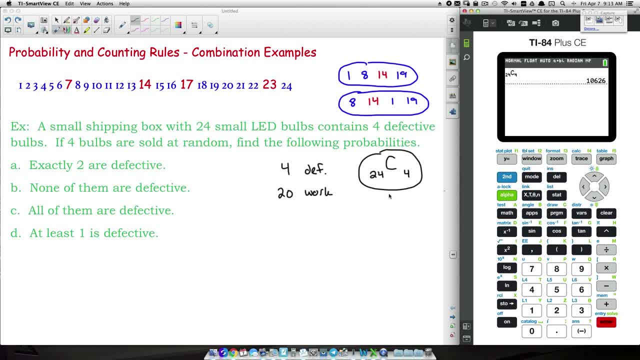 four bulbs. So we have a total of 10,626 ways, 10,626 ways that you can sell four bulbs out of 24 bulbs to a customer. And again, this right here, that's just one way, because again, order does not. 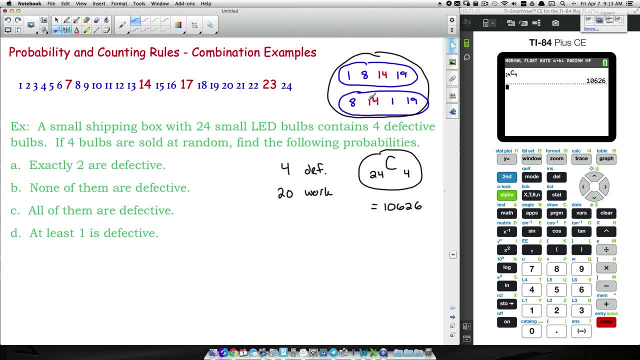 matter. in a combination We're still selling the same four bulbs. I hope that makes sense there. So how can we sell exactly two bulbs? Well, let's think about that. Question A: we're trying to sell exactly two bulbs. Question B: we're trying to sell exactly two bulbs. Question C: we're trying 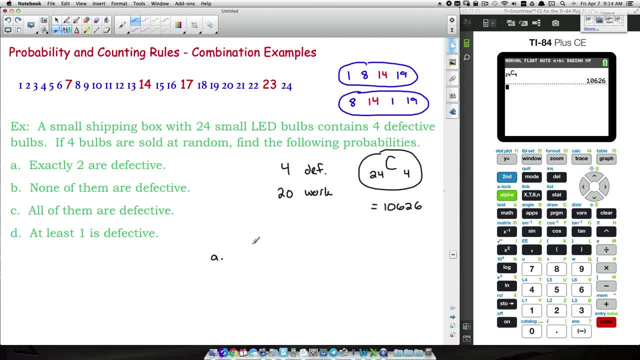 to sell exactly two bulbs. Well, let's think about this. How many ways can you do that if we look at the defective, Out of four defective bulbs, we want to choose two of them because we want exactly two. Notice I'm picking the four here. So four choose two. The reason why I'm doing that is: 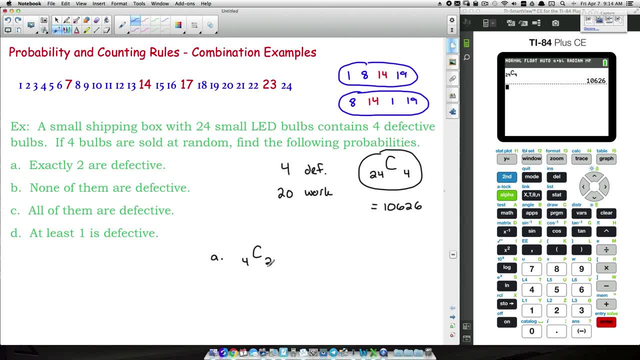 because out of the four defective, I want to choose any two of them. Now again, that would be no different if I said, okay, if I picked bulb 14 and 17,. if those were sold in a set of four, selling 14 and 17 would be the same thing as selling 17 and 14, because it's still the same. 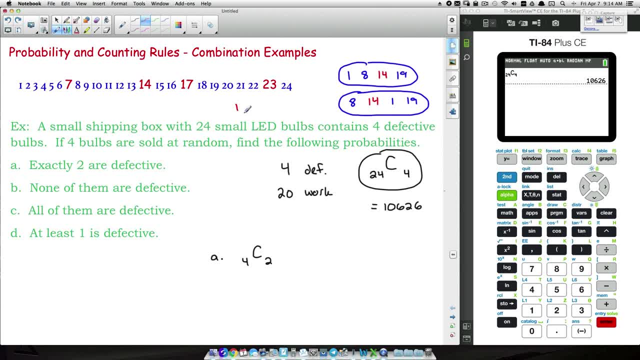 two bulbs. Order does not matter. Well, those are our two bulbs. Well, how many are we selling in all? We're selling four bulbs in all. So there's still two bulbs left that we're going to sell. So what do we do here? Well, we're selling four bulbs. Two of them are going to be defective. 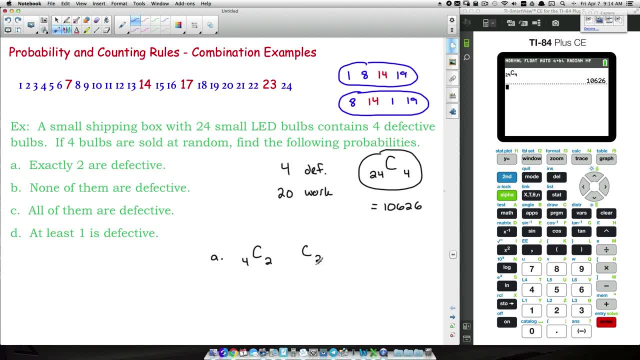 That's going to leave the remaining two that are going to be working. fine. Well, how many ways? how many are we choosing from here? It's going to be 20 working. Now think about this: Out of four of the defective, we're choosing two because we want exactly. two are defective. 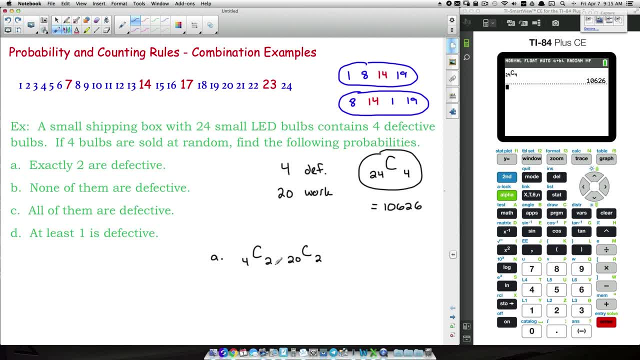 The other 20 bulbs. we want to choose two of those as well, because now, if we have two defective and two working, we do have four bulbs getting sold. So this is the number of ways that we can sell two defective and two working. And again, this is going to be out of this number right here. 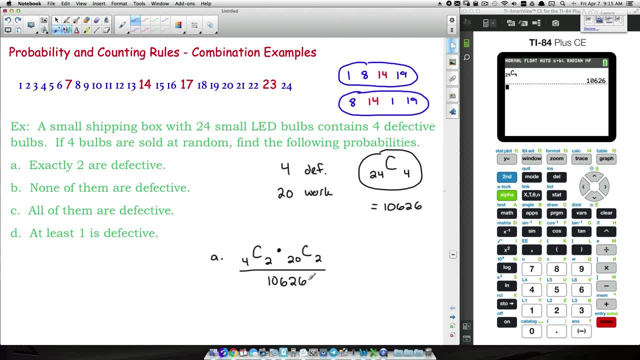 I'm just going to go ahead and write it down. So we're going to go ahead and write it down, We're going to write 10,626.. Because, remember, when you're finding probabilities, you're saying: okay, the number of ways we can do this and the number of ways we can do this, We want to multiply. 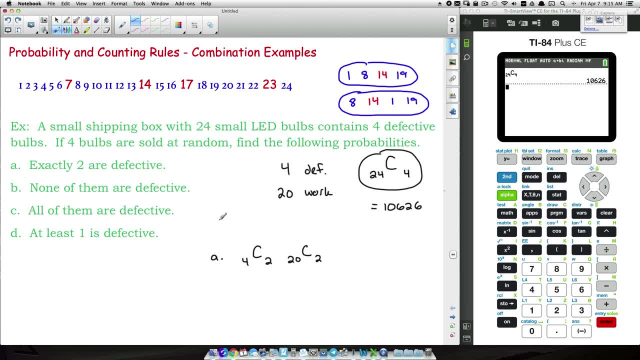 the defective. we're choosing two because we want exactly two or two are defective. The other 20 bulbs- we want to choose two of those as well, because now, if we have two defective and two working, we do have four bulbs getting sold. So this is the number of ways that we can sell two. 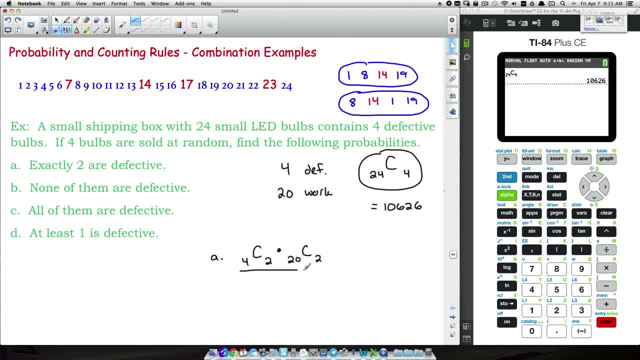 defective and two working. And again this is going to be out of this number right here And I'm just going to go ahead and write 10,000.. 626.. Because remember, when you're finding probabilities, you're saying, okay, the number. 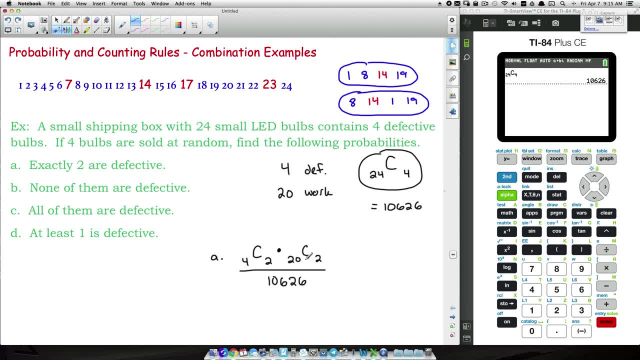 of ways we can do this and the number of ways we can do this, we want to multiply those together. So let's go ahead and do that in our TI-84 right now. So four choose two, and then we're going to. 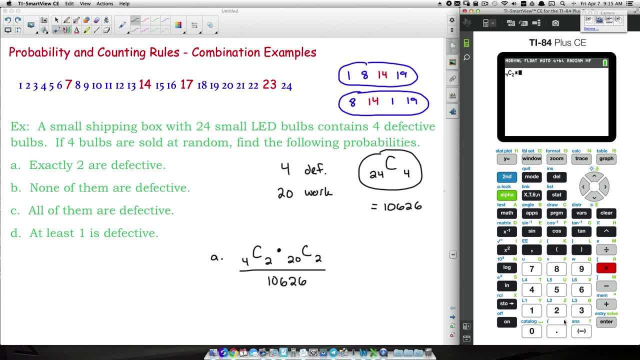 multiply- Make sure you get out of your little subscript thing down there- And 20, choose two. And then we want to divide This by the 10,626, because again, that's a total number of ways that we can sell four bulbs out of. 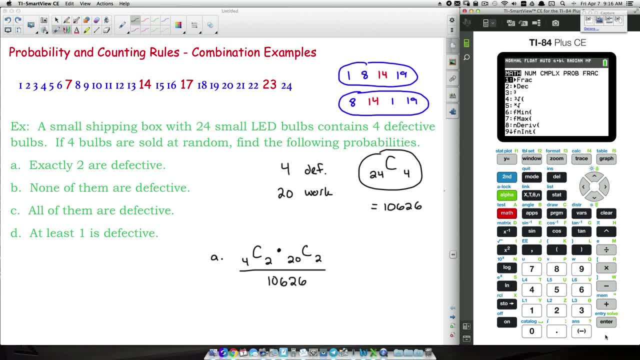 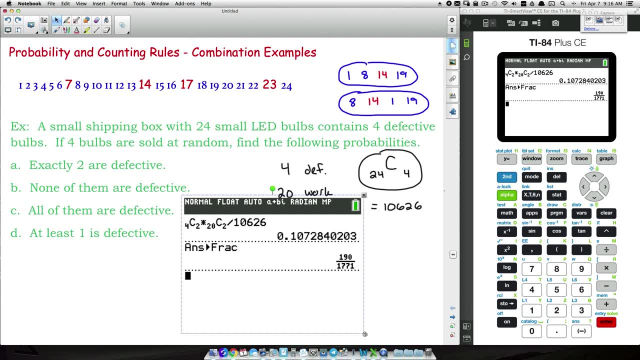 24 bulbs. So we're looking at that probability And if we convert this to a fraction, we get something like that. So this is our answer to question A. And again, this can't. it's going to take some practice, It's going. you have to make sure you understand what a combination is And 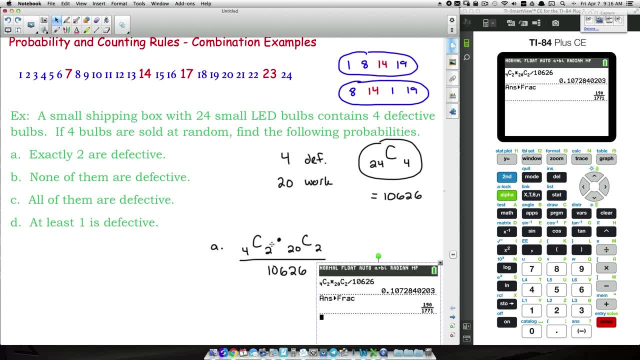 then you also got to understand your basic probability rules. when we're doing, you know we got two ways of doing this or four. choose two ways of doing this And and multiply 20,. choose two ways of doing this. right here, We multiply those together. 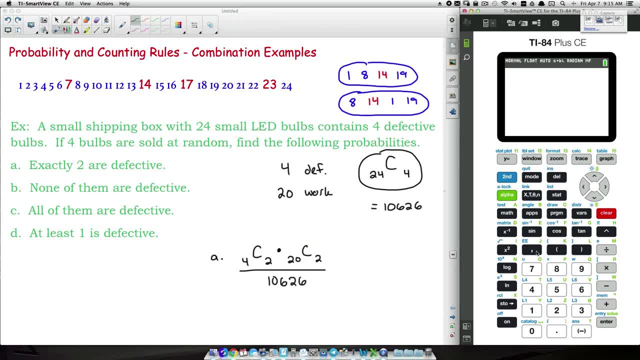 those together. So let's go ahead and do that in our TI-84 right now. So four choose two, And then we're going to multiply- Make sure you get out of your little subscript thing down there- And 20 choose two. 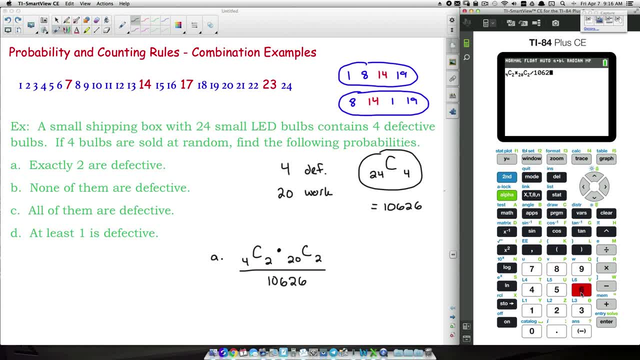 And then we want to divide this by the 10,626.. Because, again, that's the total number of ways that we can sell four bulbs out of 24 bulbs. So we're looking at that probability And if we convert this to a fraction we get something like that. So this is our answer to question A. 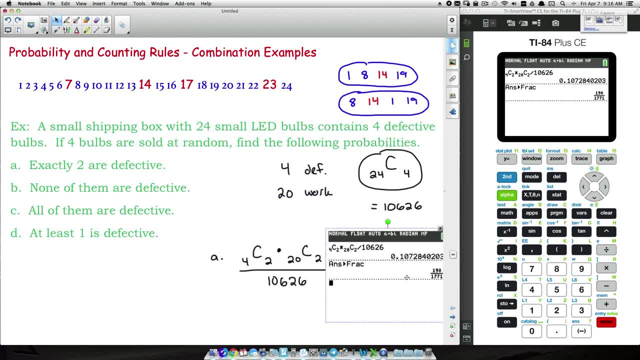 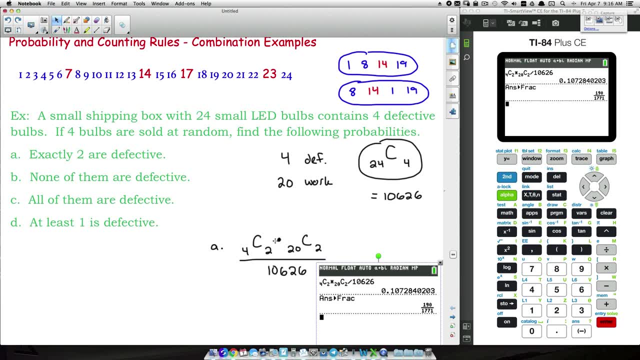 And again, this can't. it's going to take some practice, It's going. you have to make sure you understand what a combination is And then you also got to understand your basic probability rules when we're doing. you know we got two ways of doing this or four. choose two ways of doing. 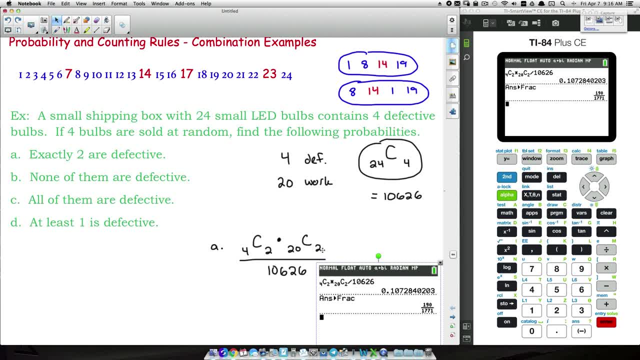 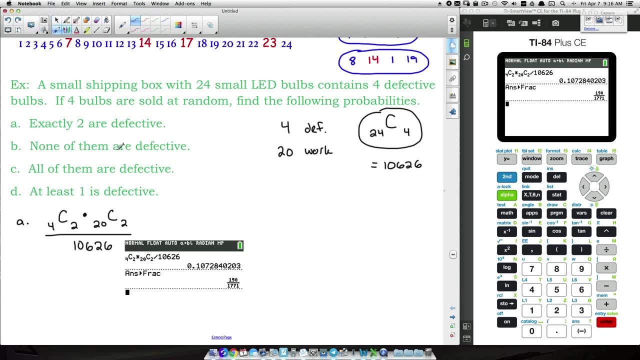 this And and multiply 20, choose two ways of doing this. right here We multiply those together, divide by the total number of ways. So that's question A. Let's look at question B now. Question B: Well, I find the probability that none of them are defective. So question B. 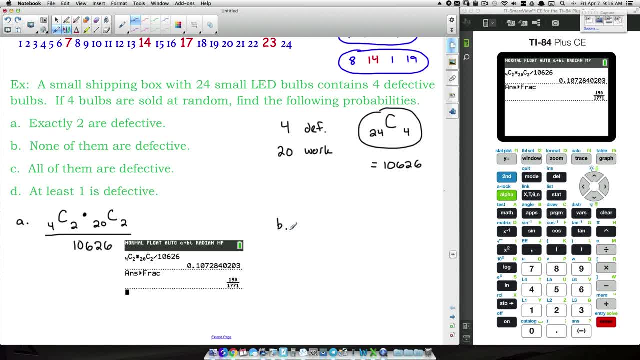 we're looking at, no bulbs are defective. Well, how in the world can we do that If no bulbs are defective? that means we're selling four bulbs that are working. Well, how many bulbs are defective? Well, how many bulbs are defective? Well, how many bulbs are defective? Well, 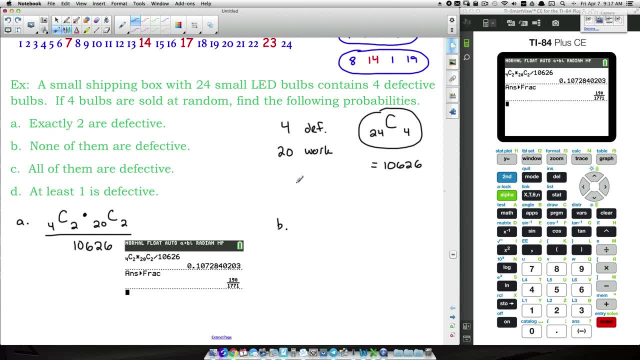 how many bulbs are working in all 20, right, We addressed that back here too And we mentioned it up here. So out of 20 working bulbs, we want to choose four, because we want all four of these bulbs that we sell. We want all four of them to be working, because we want to sell none of them. 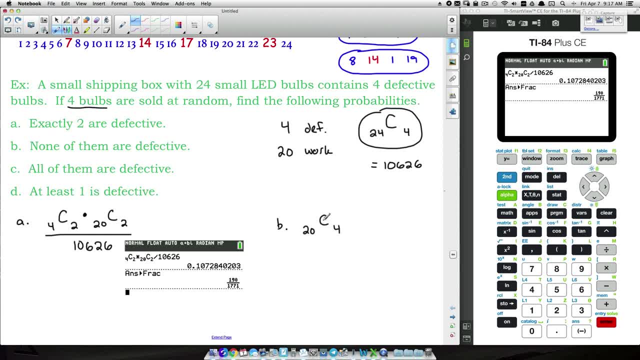 None of them are defective. So, out of 20 working bulbs, we're going to choose four working and we're going to divide this by the 10,, 6,, 2,, 6.. So let's go ahead and do that. So 20 choose four. 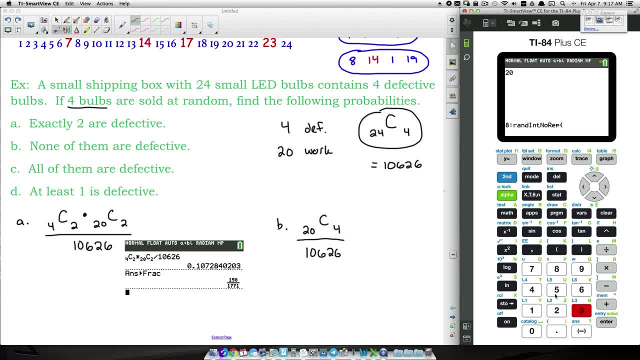 And we want to divide this by the 10,, 6,, 2,, 6.. And I'm going to go ahead and get that fraction as well. So that's our probability there. Looking here, it looks like right now we have a much. 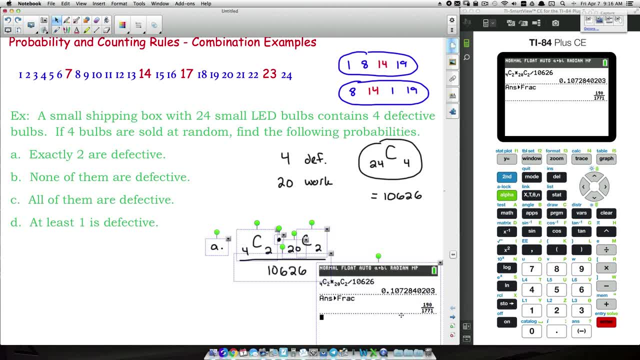 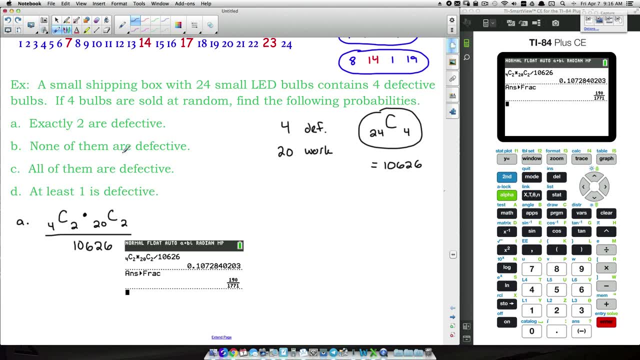 divide by the total number of ways. So that's question A. Let's look at question B now. Question B: well, I find the probability that none of them are defective. So question B we're looking at: no bulbs are defective. Well, how in the world can we do that If 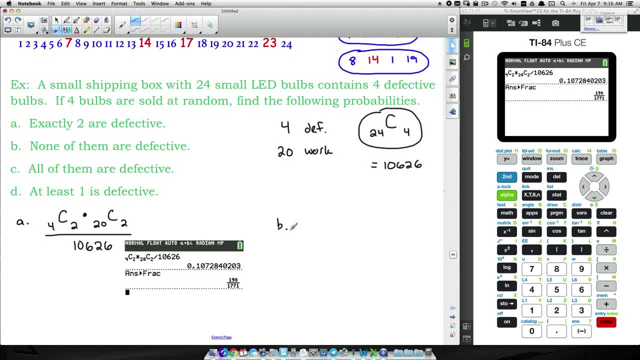 no bulbs are defective. that means we're selling four bulbs that are working. Well, how many bulbs are working in all? 20?? And then we're looking at the probability that none of them are defective. Well, right, we addressed that back here too and we mentioned it up here. so, out of 20, 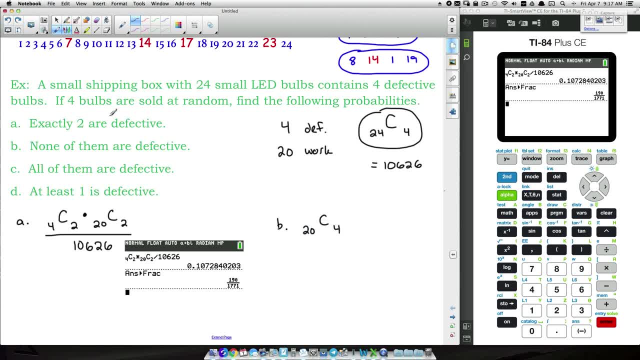 working bulbs. we want to choose four because we want all four of these bulbs that we sell. we want all four of them to be working because we want to sell none of them. none of them are defective. so out of 20 working bulbs we're going to 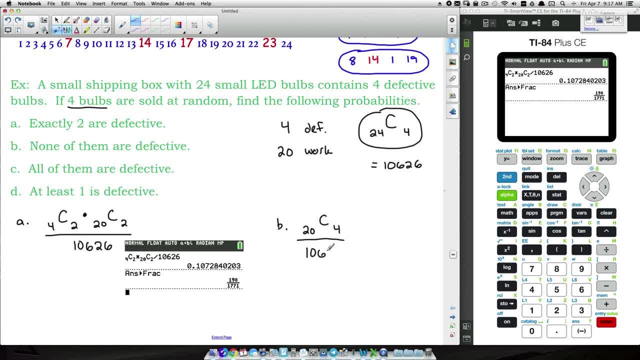 choose for working, and we're going to divide this by the 10- 6, 2, 6, so let's go ahead and do that. so 20 choose 4, and we want to divide this by the 10- 6, 2, 6, and I'm gonna go ahead and get that. 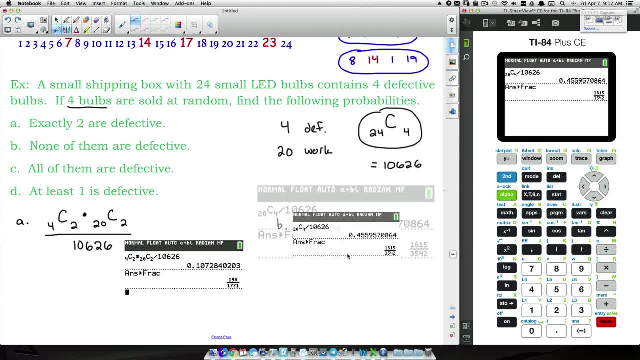 fraction as well. so that's our probability there. looking here, it looks like right now we have a much better chance of selling four working bulbs versus selling exactly two defective bulbs. look at our probability. there's only a 11% chance here and there's a 46% chance here for looking at, you know. 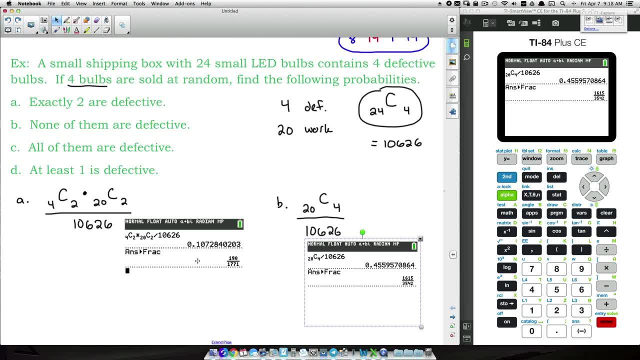 percentages or whatever. now, what's the difference between a working bulb and a non-working bulb? what's the probability of all of them being defective? well, think about this: how many bulbs are you selling? you're selling four bulbs, right? you're picking or you're choosing from 24, and out of those 24, four of them are 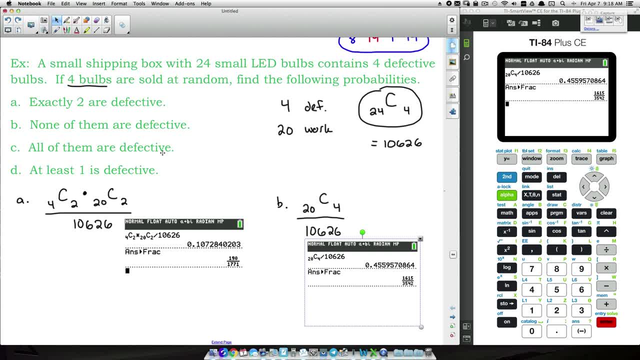 jacked up. so really, what you're going to do here, if you're going to sell all of them, if all of them are going to be defective, you're picking those four bulbs out of the 24 and imagine that's gonna be pretty hard for you to you know. 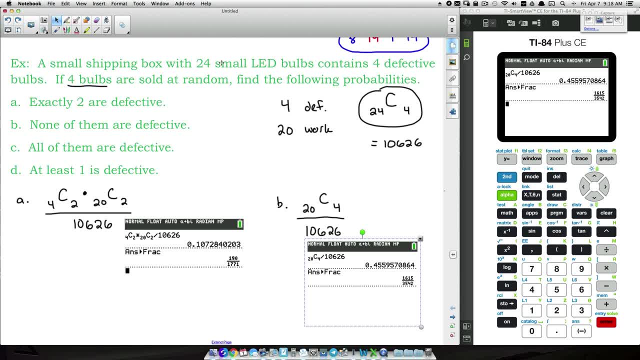 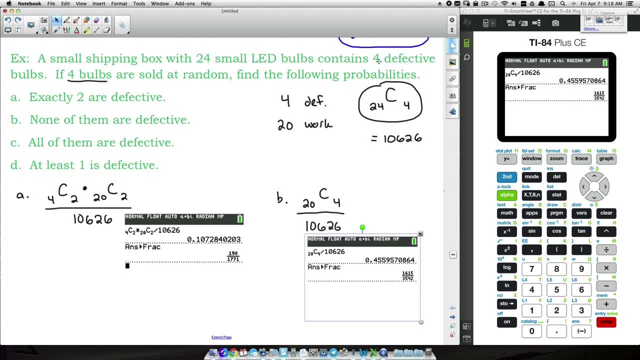 stick your hand in this box of 24 bulbs and you pick out all four defective 24 to sell. there's only one way you can do that right, because out of the four defective bulbs in your shipping box, four of them are jacked up and you're. 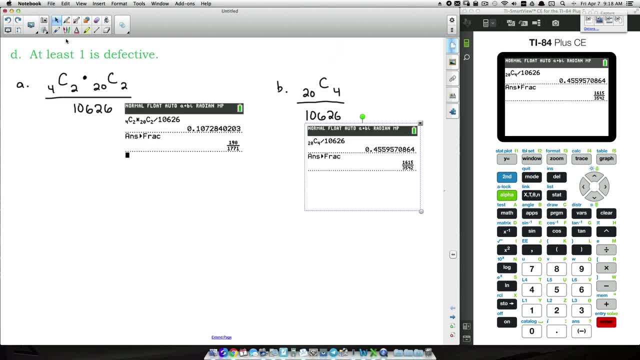 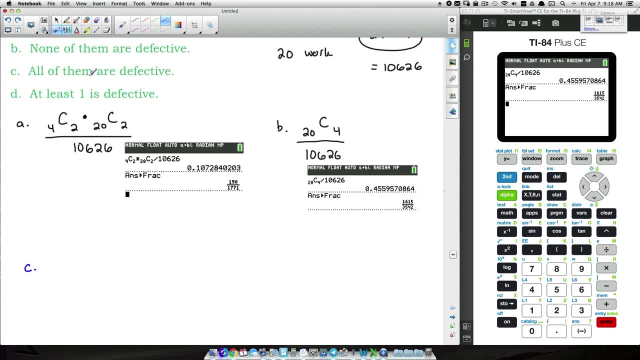 selling all four of them. so that's gonna be very unlikely. but to address that in question C, how many ways can we do this? so all of them are defective? well, out of four defective bulbs, we're going to choose all four of them and just to go. 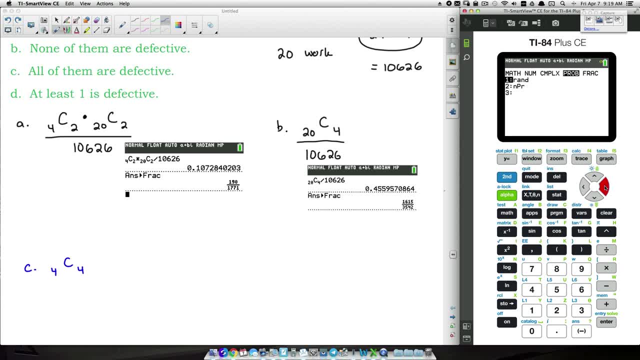 ahead and stress that to you four choose four is going to be one. there's only one way you can do that, since order does not matter. notice, we get one. so we're gonna put this over ten thousand six hundred twenty six, so therefore we have one over. 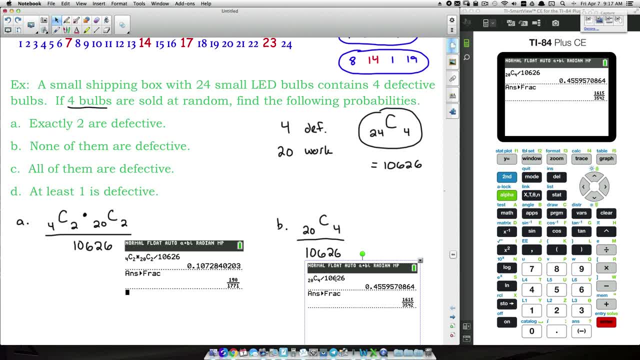 better chance of selling four working bulbs versus selling exactly two defective bulbs. Look at our probability. There's only an 11% chance here and there's a 46% chance here. So that's our probability. So that's our probability. So that's our probability. 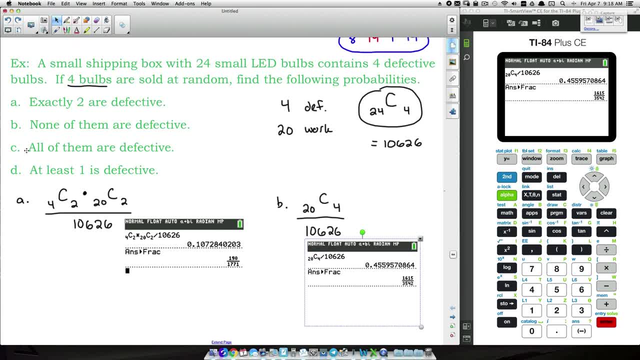 If we're looking at percentages or whatever, Now what's the probability of all of them being defective? Well, think about this: How many bulbs are you selling? You're selling four bulbs, right? You're picking or you're choosing from 24, and out of those 24,, four of them are jacked up. 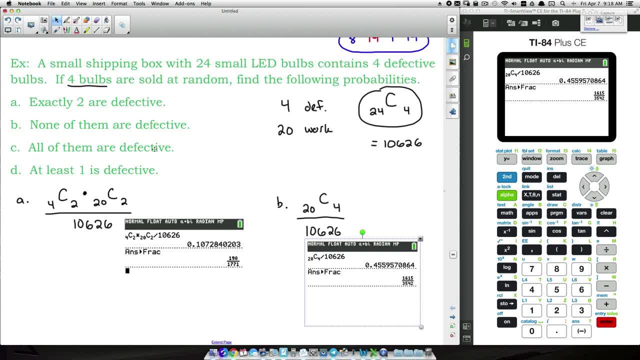 So really, what you're going to do here, if you're going to sell all of them, if all of them are going to be defective, you're picking those four bulbs out of the 24. And imagine that's going to be pretty hard for you to stick your hand in this box. 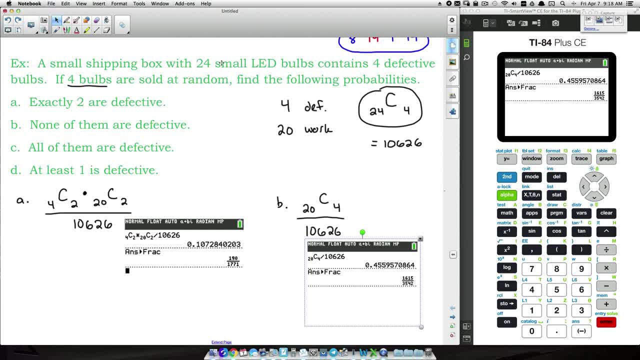 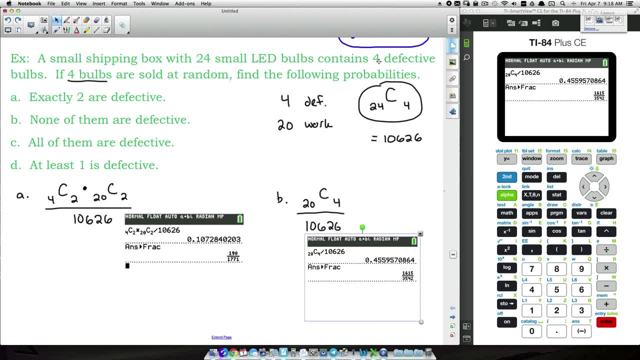 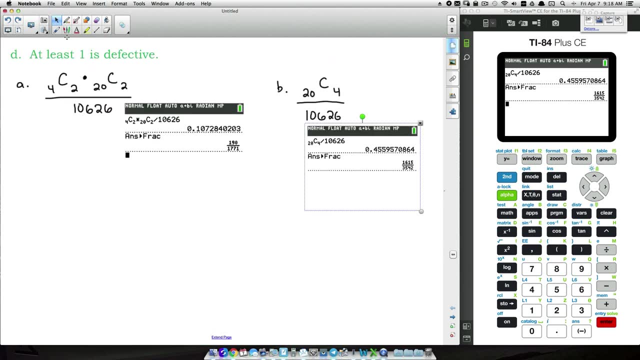 Of 24 bulbs and you pick out all four defective to sell. There's only one way you can do that right, Because out of the four defective bulbs in your shipping box, four of them are jacked up and you're selling all four of them. So that's going to be very unlikely, But to address that, 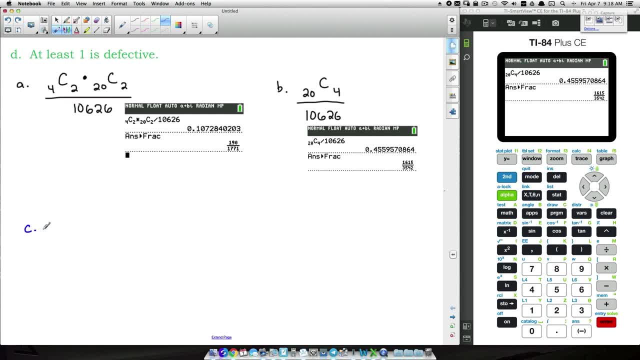 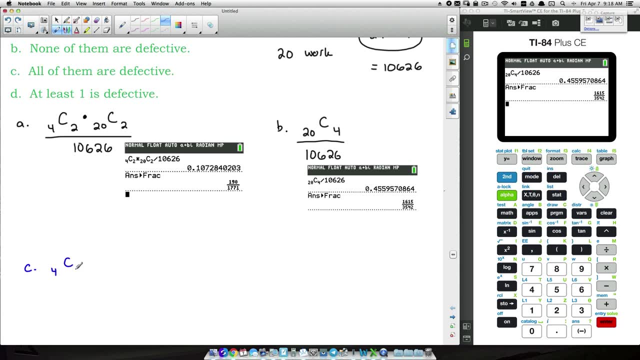 in question C. how many ways can we do this? So all of them are defective. Well, out of four defective bulbs, we're going to choose all four of them. Just to go ahead and stress that to you. four choose four is going to be one, There's only one. 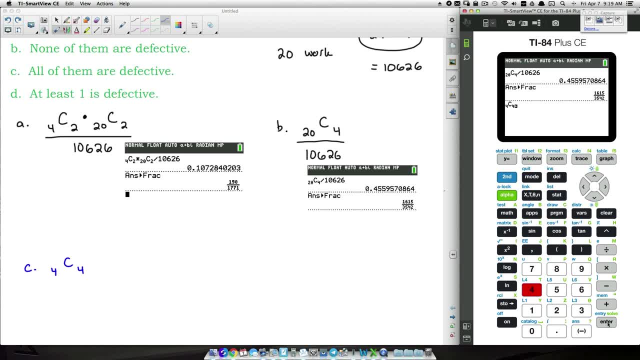 way you can do that, since order does not matter. Notice we get one, So we're going to put this over 10,626.. So therefore, we have one over 10,626.. And I'm just going to go ahead and divide that. 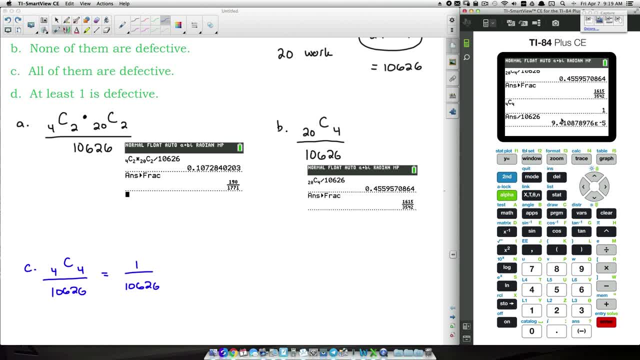 And I mean that's very unlikely, virtually impossible. I mean we're talking, you know, move that around. We're going to go ahead and divide that Decimal over E. negative five means move this decimal over five places to the left. So we're. 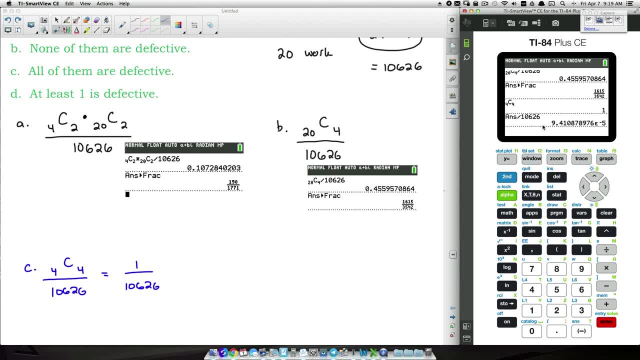 talking a fraction of a percent, not even a 1% chance, nowhere near 1% chance, Because think about that. Imagine that box filled up with 24 bulbs. four of those are jacked up and you got to pick up, you got to pick, you got to choose all four of those. It's not going to happen. 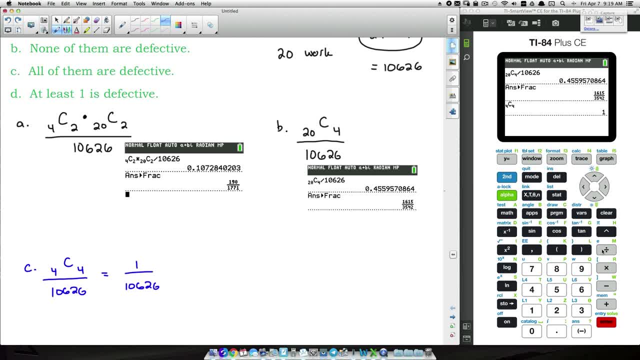 ten, six to six, and I'm just go ahead and divide that and I mean that so very unlikely, virtually impossible. I mean we're talking, you know, move that decimal over e negative five means move this decimal over five places to the left. so we're talking a fraction of a percent, not even a one percent chance. 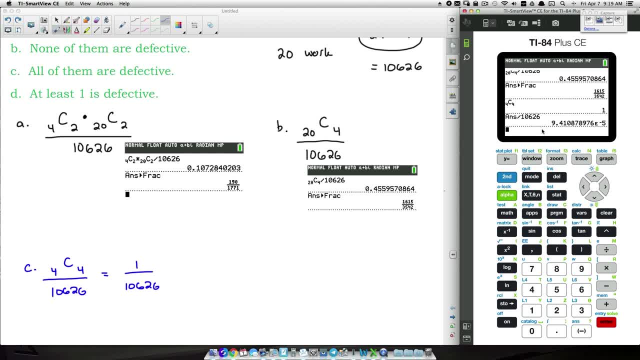 nowhere near one percent chance, because- think about that- imagine that box filled up with 24 bulbs. four of those are jacked up and you got to pick up, you got to pick, you got to choose all four of those. it's not going to happen, very unlikely. 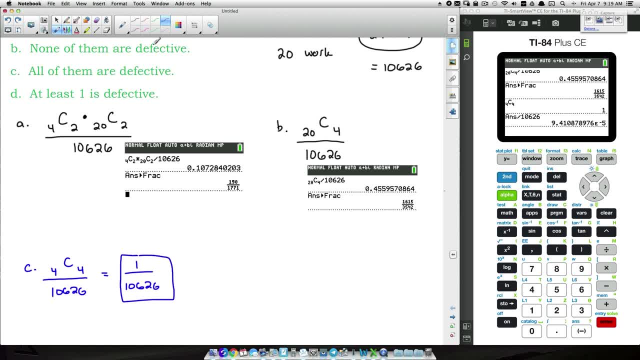 that you'll do that. so again, there's our decimal for that one, and then this last one here now. there's going to be a shortcut for this and I'm going to share that shortcut with you right here in a second. but if you want at least one defective, at least one defective means one can be. 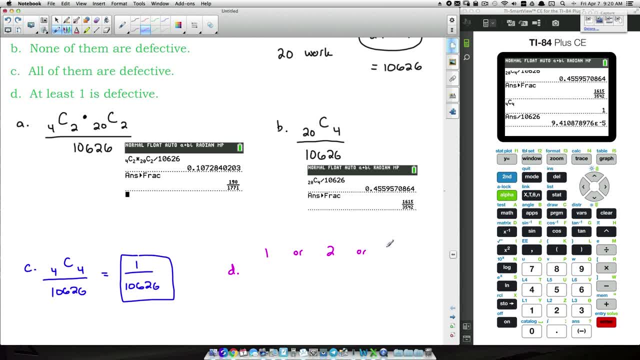 defective, or two can be defective, or three can be defective, or four can be defective, out of a total number of ten thousand six hundred and twenty six ways of choosing four bulbs from a pile of 24. so we have to address each one of these individually, and I mean so at least one, means it can be one or two, or three, or 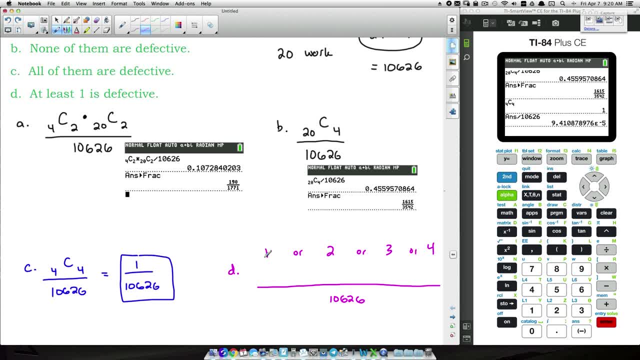 four now addressing these individually. so if one is defective, how many ways can we do that? well, let's think about it. so I'm addressing just the one bulb right now. so out of four defective bulbs, we want to choose one of those bulbs. how many are we selling? we're selling four bulbs, and all well, out of the other 20 working. 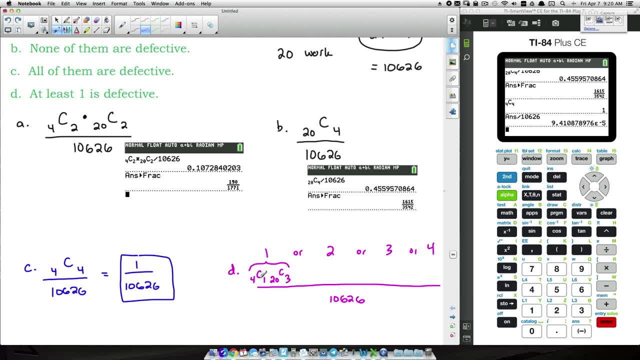 bulbs. we want to choose three of those. that is the number of ways that you can sell one defective bulb out of four defective, you're choosing just one. out of the other 20 working bulbs, you're choosing three because notice this number here and this number here represents the total number of bulbs. 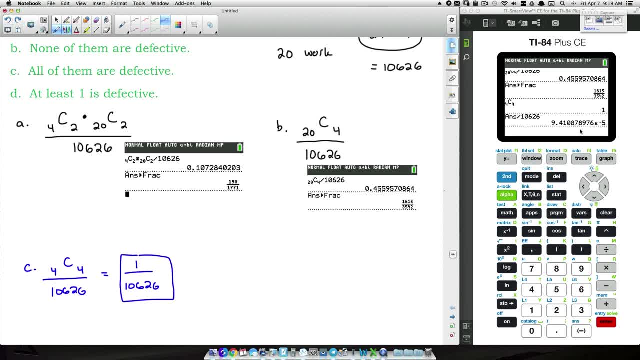 Very unlikely that you'll do that. So again there's our decimal for that one, And then this last one here. Now there's going to be a fraction of a percent. So we're going to go ahead and a shortcut for this, And I'm going to share that shortcut with you right here in a second. 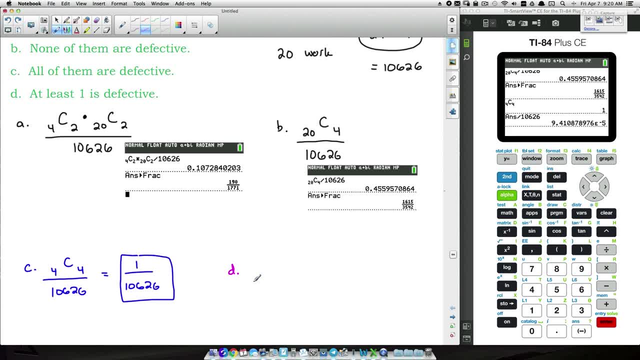 But if you want at least one defective, at least one defective means one can be defective, or two can be defective, or three can be defective, or four can be defective, Out of a total number of 10,626 ways of choosing four bulbs from a pile of 24.. So we have to address: 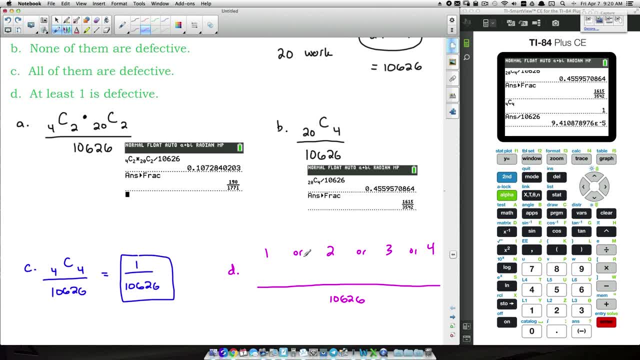 each one of these individually, And I mean so at least one means it can be one or two, or three or four, Now addressing these individually. So if one is defective, how many ways can we do that? Well, let's think about it. 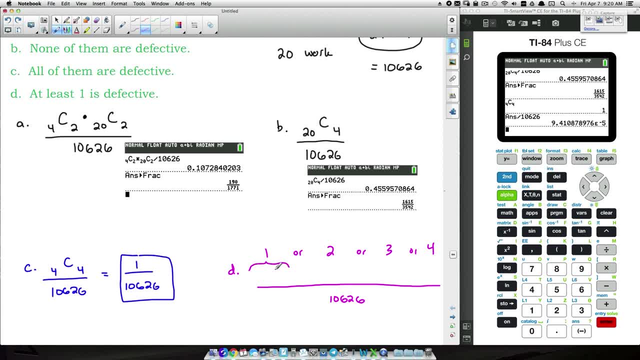 So I'm addressing just the one bulb right now. So, out of four defective bulbs, we want to choose one of those bulbs. How many are we selling? We're selling four bulbs in all. Well, out of the other 20 working bulbs, we're going to choose one of those bulbs. So we're going to choose one of those. 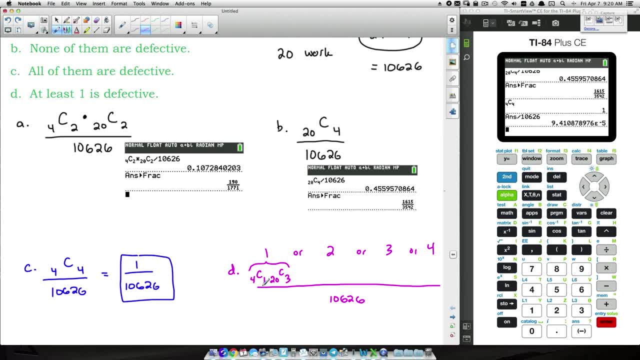 bulbs, So we want to choose three of those. That is the number of ways that you can sell one defective bulb. Out of four defective, you're choosing just one. Out of the other 20 working bulbs, you're choosing three because- notice this number here, and this number here represents the 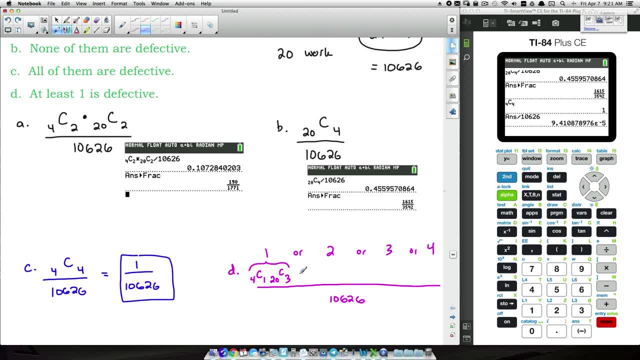 total number of bulbs you're selling in all, All right, Or plus. now let's do two. So out of four defective bulbs, you're going to now choose two, because we're looking at a scenario of two defective. And then what are we going to multiply that by? Well, the remaining 20. 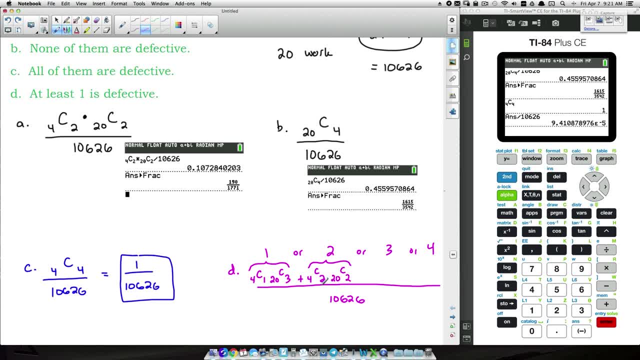 that we have. we want to choose two of those as well, because we're selling four bulbs. Two plus two is four, So we're selling two defective two of the working ones, Or is plus. So now coming to here, Out of four defective bulbs, Okay, We're looking at selling three. now We're going to. 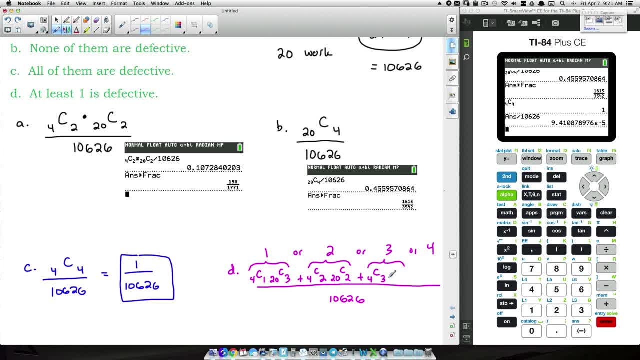 choose three And then out of your 20 working bulbs you're going to choose one of those bulbs. We're going to choose one because now again we're selling three defective, which means we're going to sell one working bulb because we're selling four bulbs in all. Let me move that back. 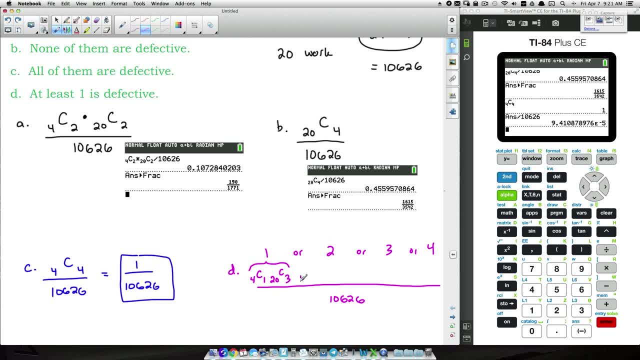 you're selling in all, all right, or plus, now let's do two. so, out of four defective bulbs, you're going to now choose two, because we're looking at the scenario of two defective, and then what are we gonna multiply that by well, the remaining 20 that we have. we want to choose two of those as well, because 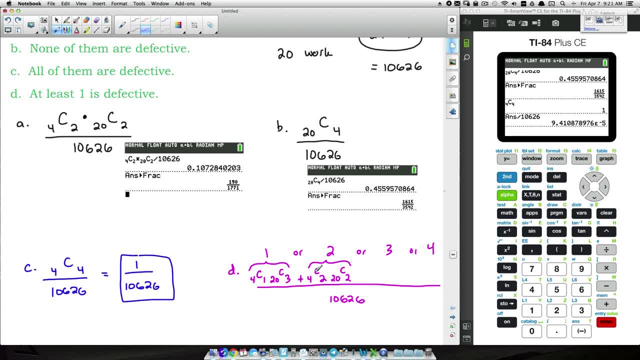 we're selling four bulbs. two plus two is four. so we're selling two defective two of the working ones, or is plus. so now coming to here, out of four defective bulbs, okay, we're looking at selling three. now we're going to choose three and then, out of your 20 working bulbs, you're going to choose one, because now 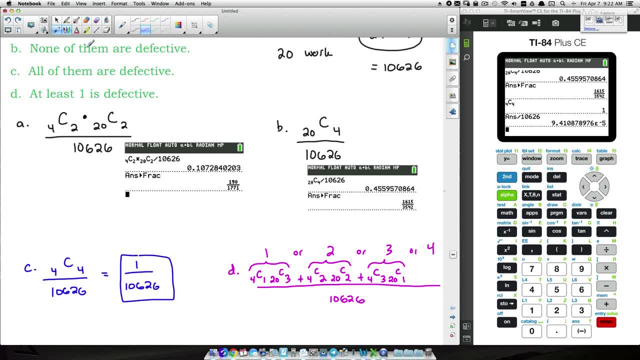 again, we're selling three defective, which means we're going to sell one working bulb because we're selling four bulbs in all. Let me move that back. I'm just trying to try to slide this over a little bit and get some room. And then our last scenario- we've actually already addressed that- And to be 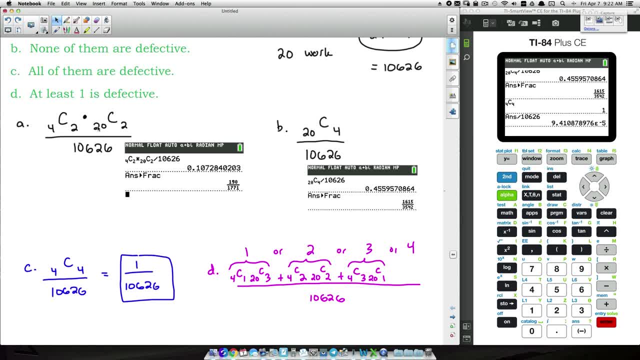 quite honest with you. we've already addressed this two deal as well. That was the one we did up here- Notice that that's the same deal right there- And then this last piece down here. So four: we've already addressed that. That was this one over here. but just to kind of look at it and 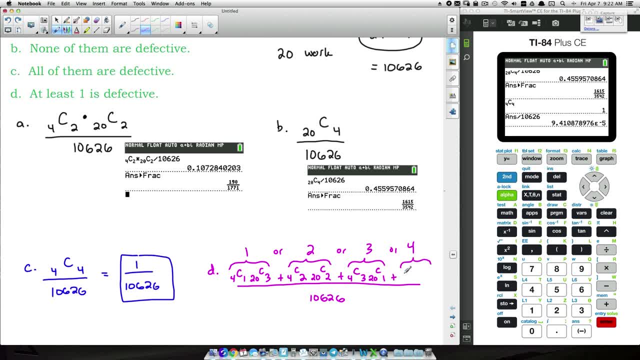 maybe explain some other ideas of combinations to you. So we want to sell four defective. So out of four defective, we're going to choose all four, because we're looking at the scenario of selling four defective bulbs. Well then, out of the other 20 working bulbs, we don't want to choose any of. 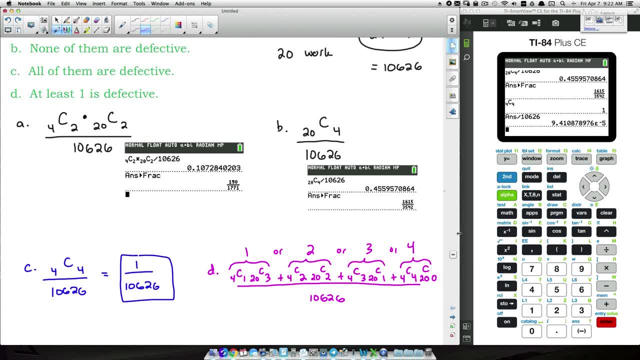 those, because we're selling four bulbs and we want all four of them to be defective in this scenario. So again, at least one- means one or two or three or four- could be defective. Now, that's a lot of work. So we're going to look at that scenario and we're going to look at the scenario. 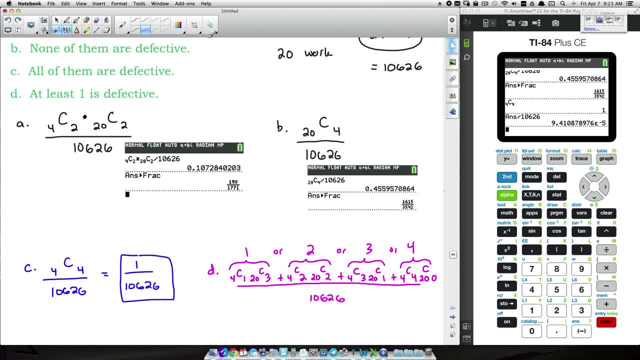 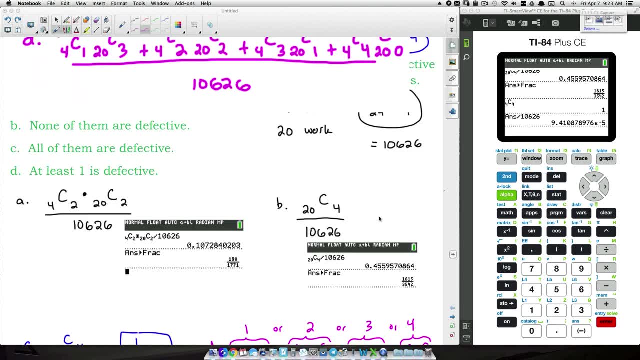 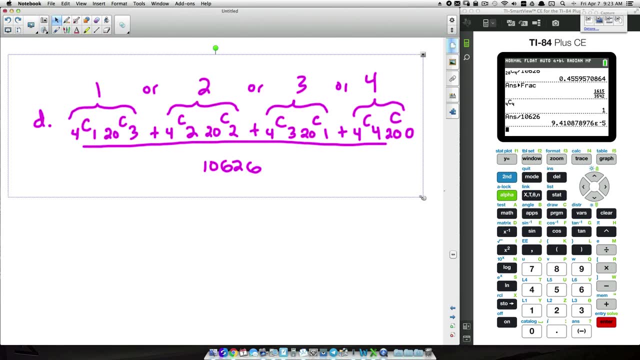 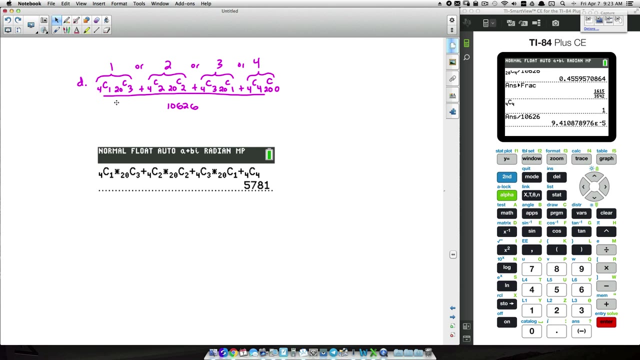 lot to type in. so what I've uh went ahead and done here is: I'm just going to take this and we're going to put that over on another page, because I've already uh got this worked out earlier. so, out of 10,626 possible ways to sell four bulbs for out of 24 bulbs, um, that's that. 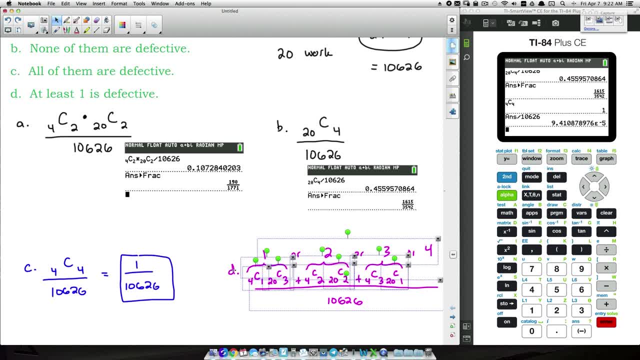 I'm just trying to slide this over a little bit and get some room. And then our last scenario. we've actually already addressed that And, to be quite honest with you, we've already addressed this two deal as well. That was the one we did up here. Notice that That's the same deal, right? 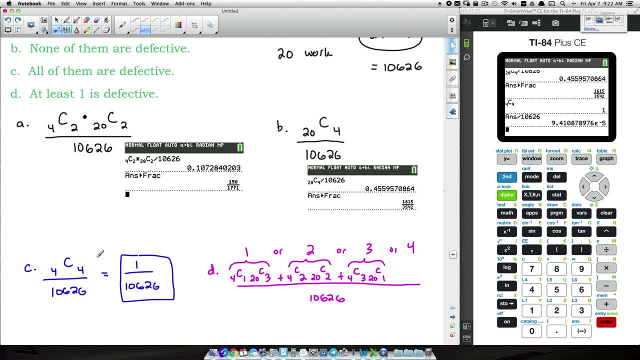 there And then this last piece down here, So four. we've already addressed that. That was this one, just to kind of look at it and maybe explain some other ideas of combinations to you. So out of we want to sell four defective. So out of four defective we're going to choose all four. 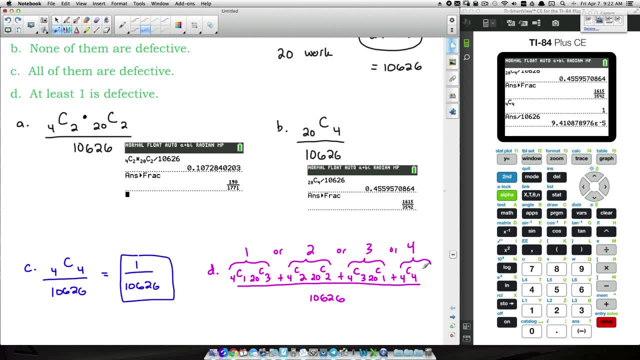 because we're looking at this scenario of selling four defective bulbs. Well then, out of the other 20 working bulbs, we don't want to choose any of those, because we're selling four bulbs and we want all four of them to be defective in this scenario. So, again, at least one means one, or two, or three. 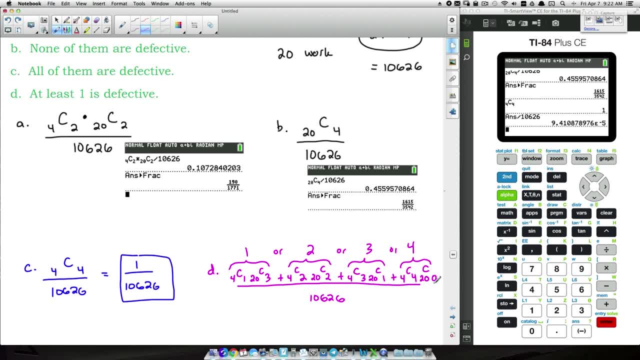 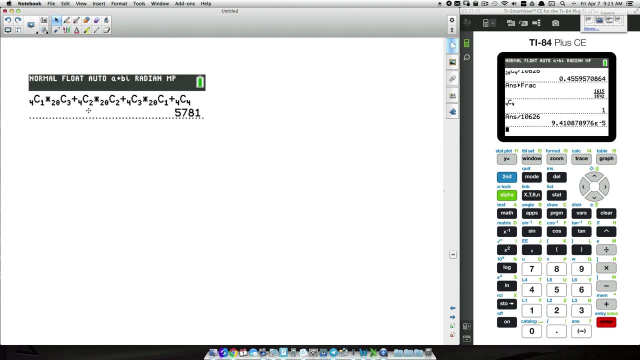 or four Defective. Now that's a lot to type in. So what I've went ahead and done here is: I'm just going to take this and we're going to put that over on another page because I've already got this worked out earlier. So, out of 10,626 possible ways to sell four bulbs for out of 24 bulbs, that's that. 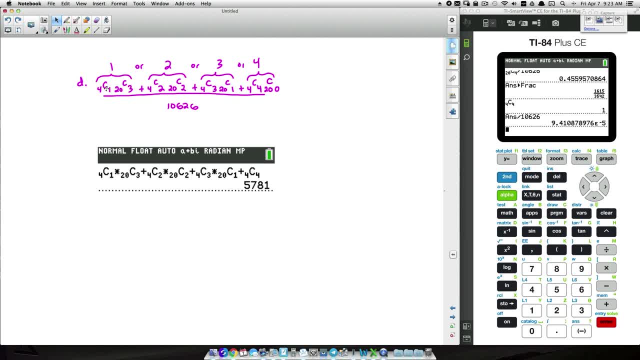 10,626 ways. But out of doing that, if you look at what I've wrote here. so four choose one, 20 choose three. I'm matching these up: four choose two, 20 choose two, four choose three, 20 choose one, and then four choose four. Now you might say: 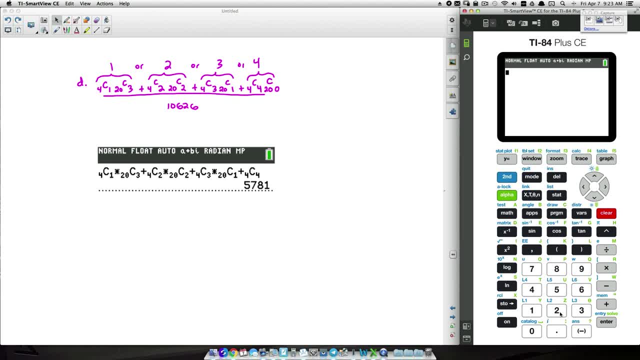 oh, I left this off. Well, that's no big deal, because 20 choose zero. what is that going to be? 20 choose none- What's that going to be? That's going to be one. So I mean really this times one. 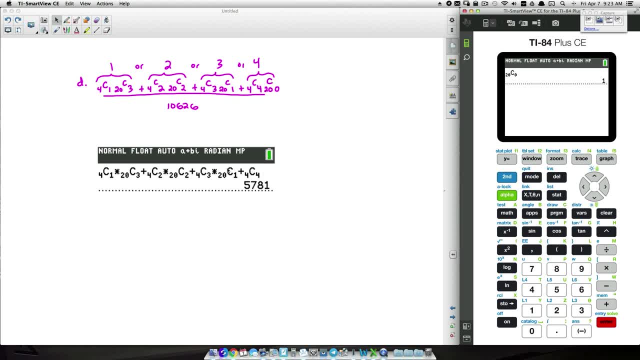 is still going to be just that. So that's what I have right there. So that's going to be our numerator. all that stuff right there, That's going to be our numerator. That's 5,781 ways out of 10,626 ways. Well, let's see what we. 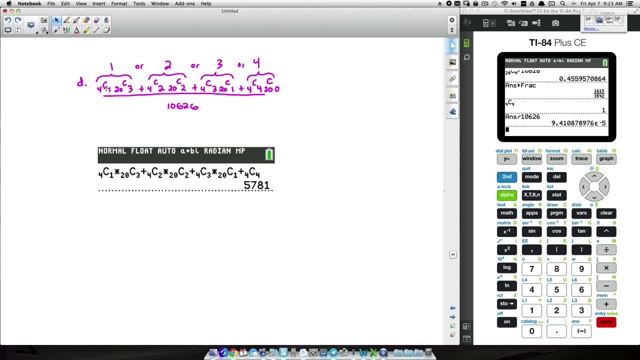 10,626 ways. but out of doing that, if you look at what I've wrote here: so four choose one, 20 choose three. I'm matching these up: four choose two, 20 choose two, four choose three, 20 choose one, and then four choose four. now you might say: oh, I left this off. well, that's no big deal, because 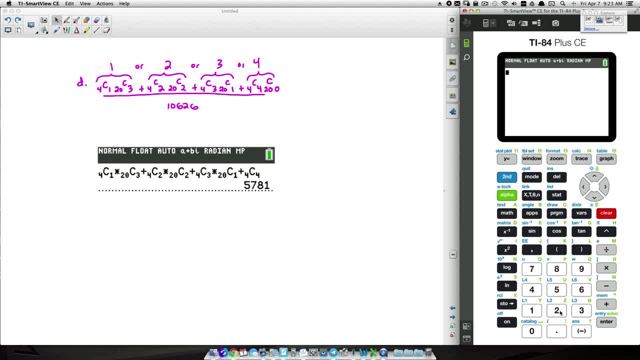 uh, 20 choose zero, what is that going to be? 20 choose none- what's that going to be? that's going to be one. so I mean, really, this times one is still going to be just that. so that's what I have right there. so that's going to be our numerator. all that stuff right there is going to be our. 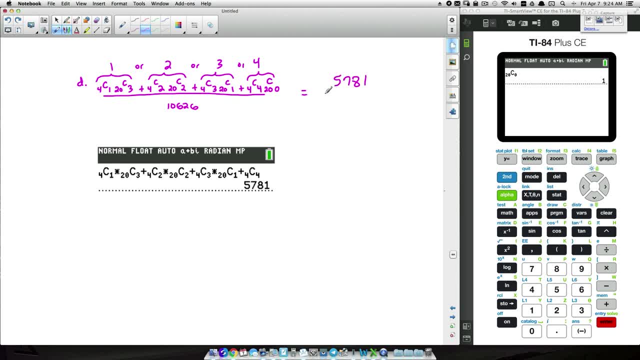 numerator, that's 5,781 ways out of 10,626 ways. well, let's see what we get there: 5781 divided by 10,626. I don't think this is going to simplify. uh, okay, yes, it did. 1927 um over 3542. so yes, it does simplify. that's the same probability as this. 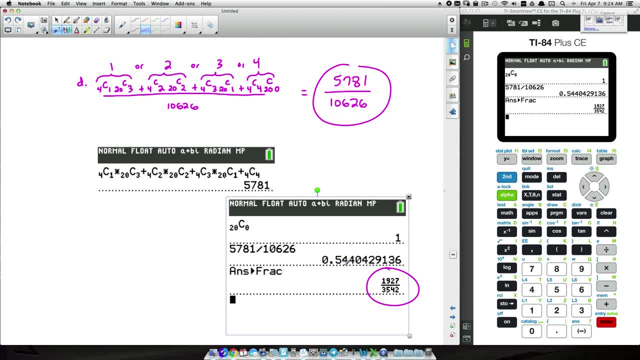 so we have a 54% chance to sell four bulbs for out of 24 bulbs for out of 24 bulbs for out of 24 bulbs for out of 25% chance of doing this. I mean that makes sense because you have a whole bunch of different. 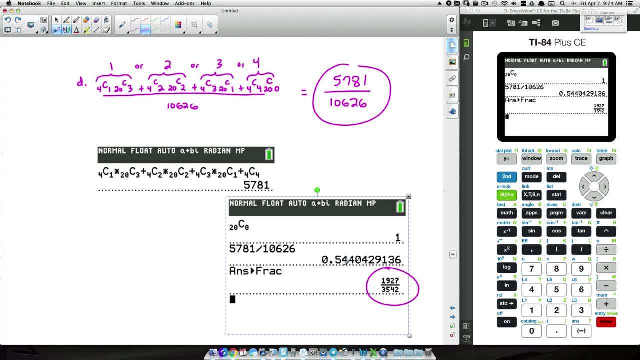 scenarios you could at least. one means, um, you could sell one defective bulb to a customer out of the four you sold them. or you could sell two defective bulbs out of the four you sold them, or three or four. so you have, you know, various probabilities getting added together with that. 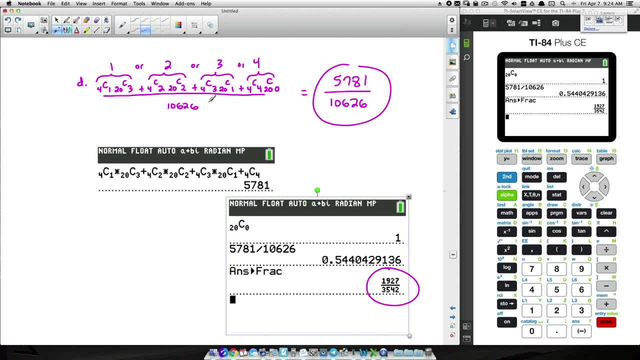 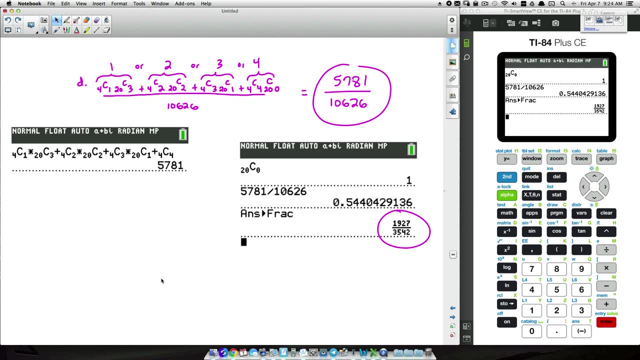 or statement. now, what's another way we could approach this? if you want at least one- and here's the shortcut- here's the shortcut for this problem- if you're going to sell at least one, that's going to be the complement of you selling no defective. think about that. if you're 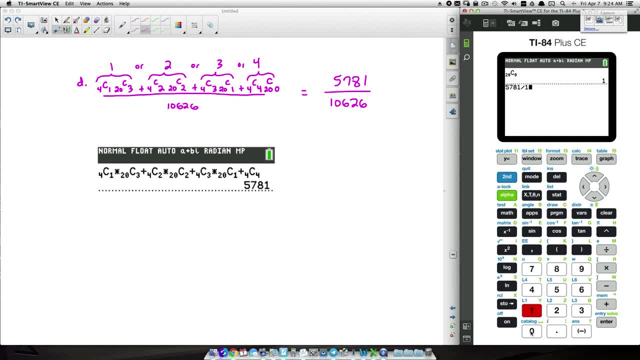 get there: 5781 divided by 10,626.. I don't think this is going to simplify. Okay, Yes, it did: 1927 over 3542.. So, yes, it does simplify. That's the same probability as this. So 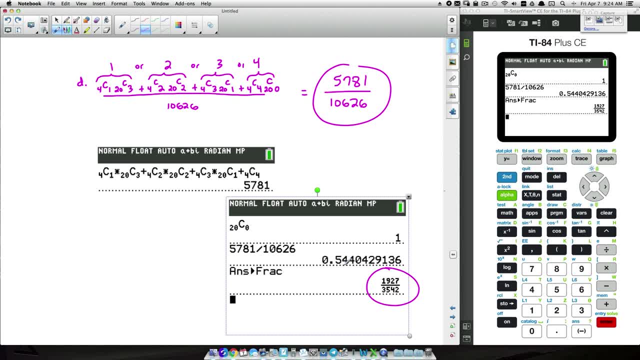 we have a 54% chance of doing this. I mean that makes sense because you have a whole whole bunch of different scenarios You could say at least one means you could sell one defective bulb to a customer out of the four. you sold them. or you could sell two defective bulbs out of the. 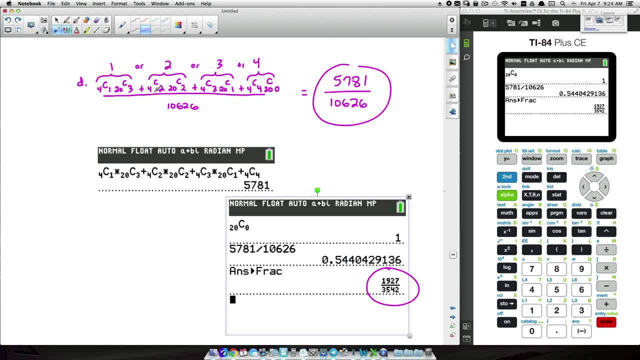 four, you sold them, or three or four, So you have, you know, various probabilities getting added together with that or statement. Now, what's another way we could approach this, If you want at least one, and here's the shortcut, here's a shortcut for this problem. If you're going to sell, 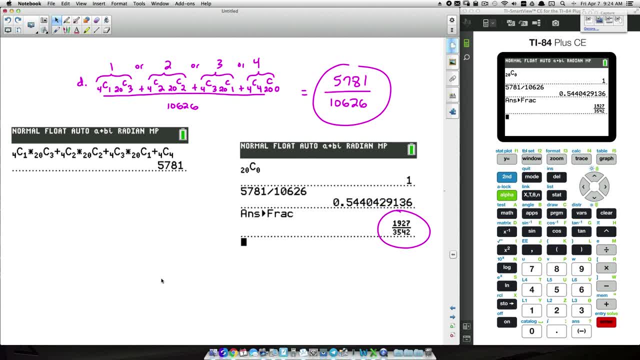 at least one. that's going to be the compliment Of you selling no defective. Think about that. If you're going to sell at least one, that means you can sell one or two or three or four. And we're selling four bulbs. Well, the only other thing. 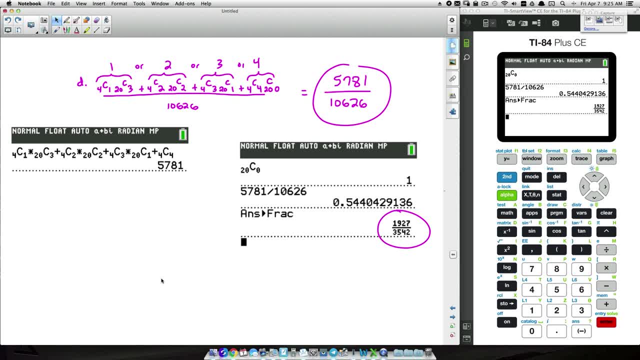 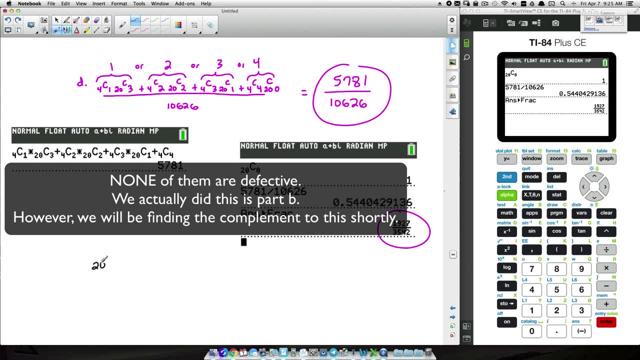 that it can't be is going to be you selling all four bulbs to a customer that work. So let's think about that. Here's a shortcut. Let's look at this scenario. Let's say, okay, out of our 20 working. 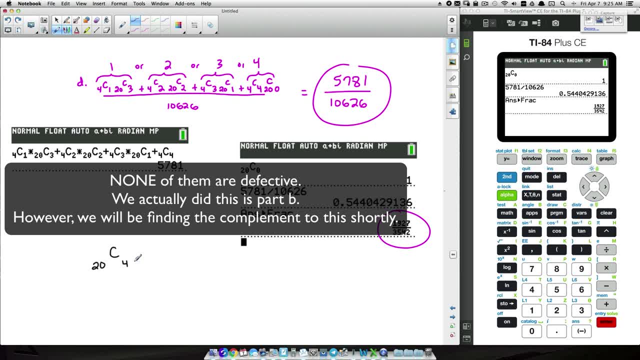 bulbs. suppose we chose all four of the bulbs that we sold out of those 20 working ones. Suppose we chose all four working ones to sell to a customer. So that's going to be the compliment. Now, if you're going to sell to a customer, let's find this probability. So 20 choose four, So 4,845.. So 4,845. 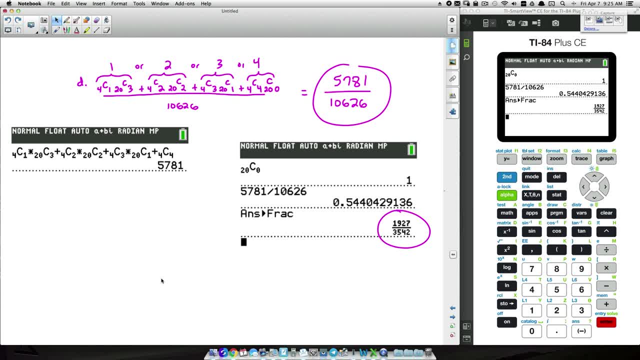 going to sell at least one. that means you can sell one or two, or three or four, and we're selling four bulbs. well, the only other thing that it can't be is going to be you selling all four bulbs to a customer. that work. so let's think about that. here's a shortcut. let's look at this scenario. let's say: 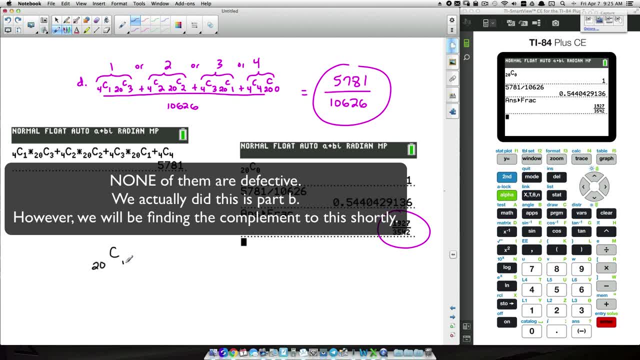 okay, out of our 20 working bulbs, suppose we chose all four the bulbs that we sold. out of those 20 working ones, suppose we chose all four working ones to sell to a customer. let's find this probability. so 20 choose four, so 4845. so 4845 over ten, six, two, six. now this ain't now watch. 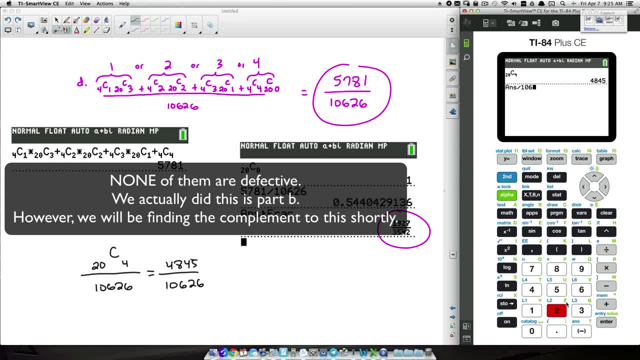 we're going. we had to talk a little bit more about this. so divide by ten, six, two, six, and we get this probability here. now, this is the only scenario that does not meet. this, at least one again means you can sell one or two or three or four defective. the only thing that's not being 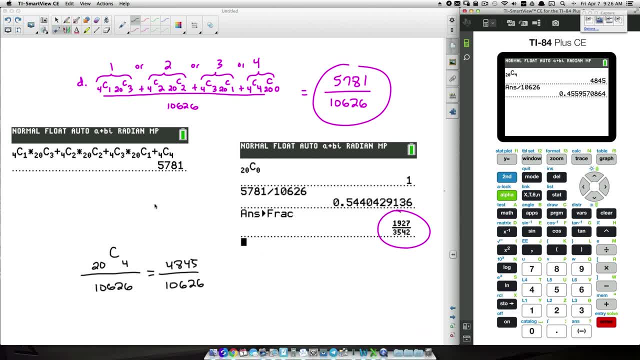 talked about here is you selling all four bulbs that are working. this is the probability of you selling all four bulbs that are working, and this is the only other scenario that could happen. so what we want to do is do the complement of this. if we take one and subtract that, answer that we 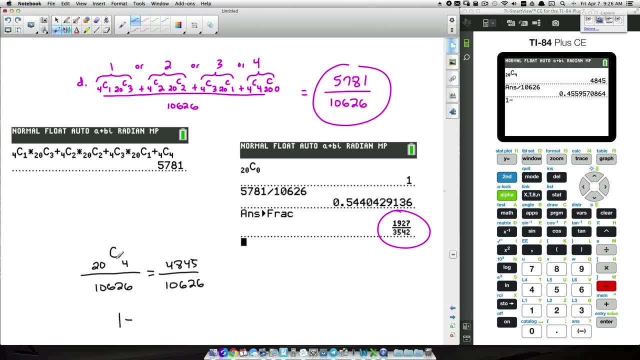 actually what we're doing here is we're taking uh, one minus that thing to find the same answer here. uh, or that answer. they are simplified, so let's take one and let's subtract that probability of four, eight, four, five over ten, six, two, six. now this is a much faster way, but it's often overlooked. 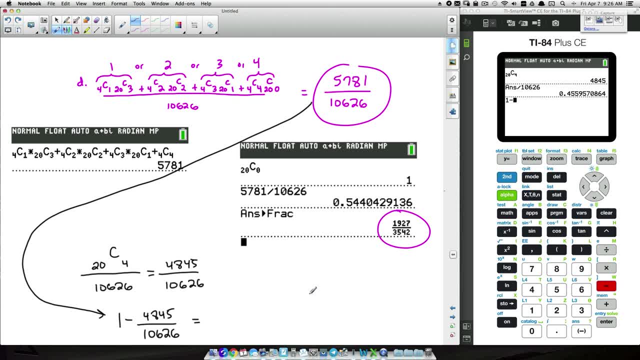 because you're not realizing that there's only one scenario where this can't happen. so divide or subtract that answer boom. and if I convert this- or maybe you remember right there, look. so we're taking one and we're subtracting the probability of us selling all four bulbs working all right. so again, that's a way you can. 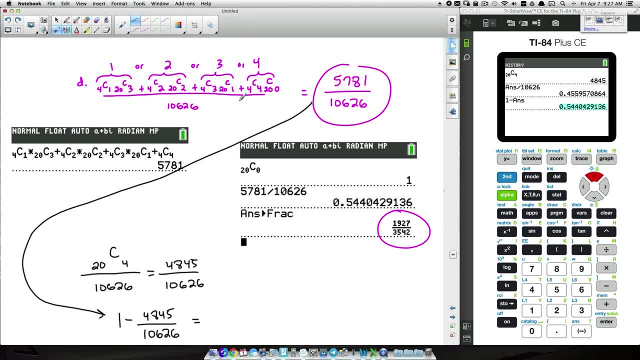 do it and typically that you will see that in a statistics course. uh, you want to take that shortcut versus you doing all this, because imagine if we had, you know, a bigger box of bulbs and we were selling more of them. you know that this will get real tedious um to do all this, so at least one. 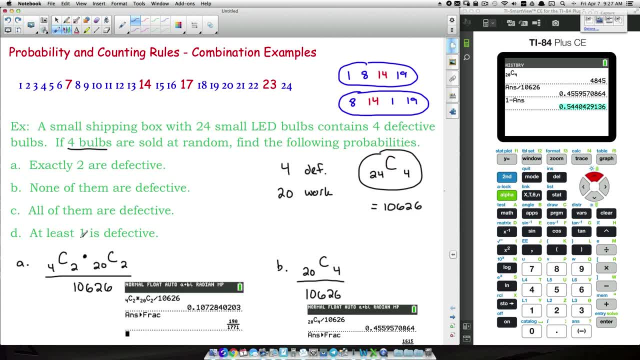 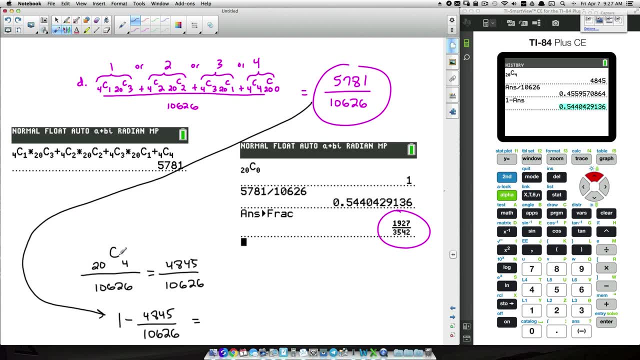 is a common uh time to say hey, let me consider the compliment. at least one, the opposite of at least one, is doing none, selling no defective. and that's exactly what I addressed right here, because out of 20 working bulbs, we could choose all four that we sell to be from the working part and that's going. 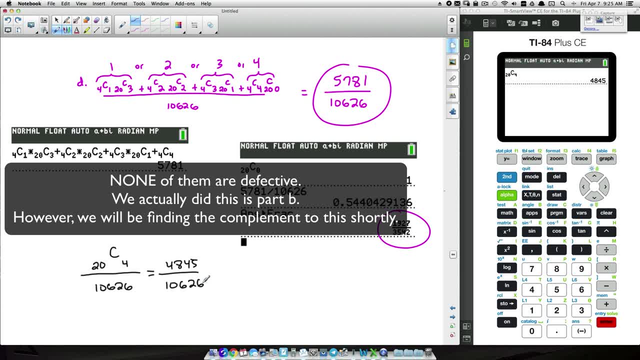 over 10,, 6,, 2, 6.. Now, this ain't now watch we're going to. we had to talk a little bit more about this. So divide by 10,, 6,, 2,, 6, and we get this probability here. Now, this is the only. 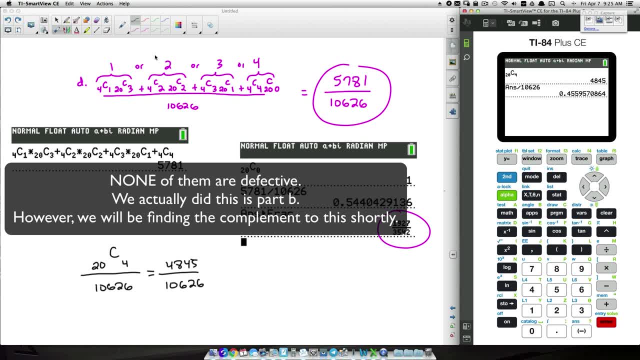 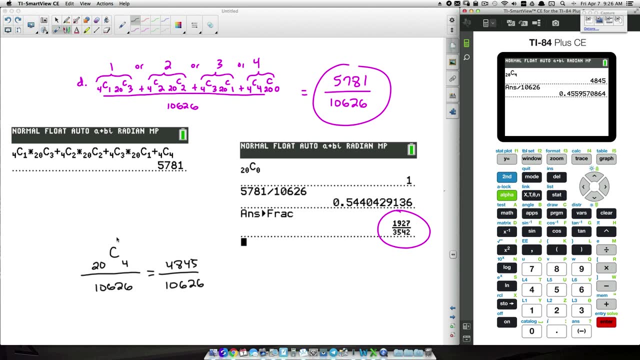 scenario that does not meet this, At least one- again means you can sell one or two or three or four defective. The only thing that's not being talked about here is you selling all four bulbs that are working. This is the probability of you selling all four bulbs that are working And this